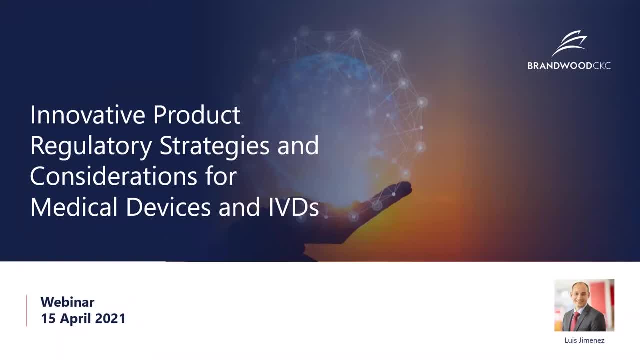 Welcome to today's webinar for BrownWood CKC. This webinar is released on April 15, 2021, and it will be focused on innovative product regulatory strategies and considerations for medical devices and diagnostics. My name is Luis Jimenez and I'll be your presenter today. 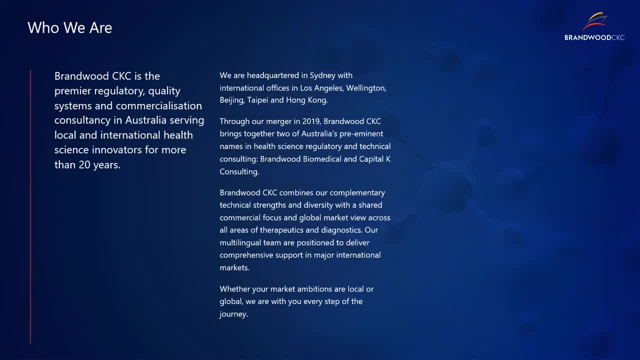 For those who might not know, BrownWood CKC is an international regulatory and quality consulting firm. Our headquarters are in Sydney, Australia, and we bring a global perspective to medical device regulatory and quality consulting. Our team combines complementary technical strengths and diversity with a shared commercial focus and global market to view all areas. 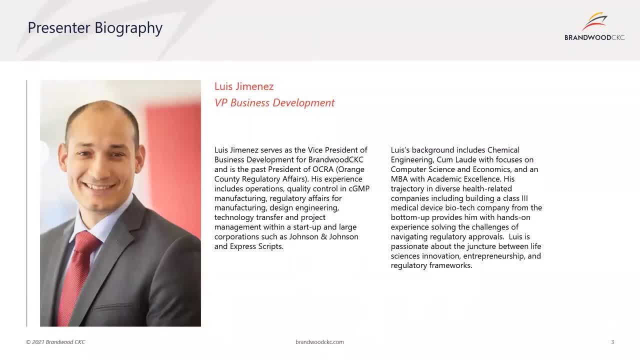 of therapeutics and diagnostics. A little bit about myself. I'm the VP of business development. I have over 12 years of experience both running a startup company and, too. And and a little bit about myself. I'm the VP of business development and I have over 12 years of experience both running a startup company and a little bin, And. 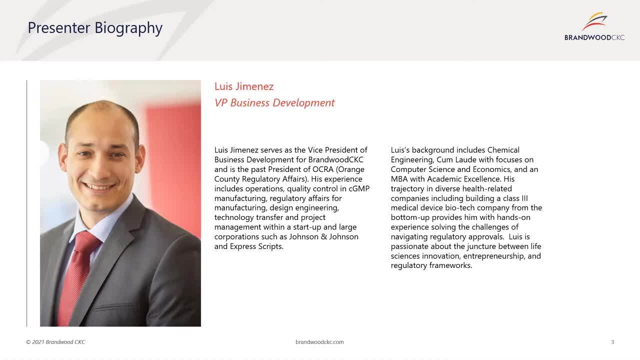 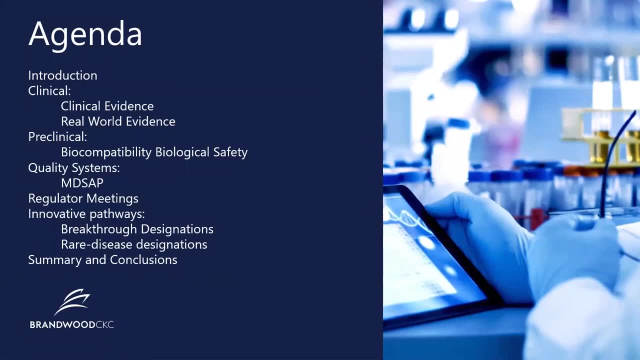 running a startup company and a little bin And working for large organizations in GMP manufacturing, regulatory affairs, project management and program management. Our agenda for today will cover a lot. We'll first start with the clinical considerations, both in clinical evidence: 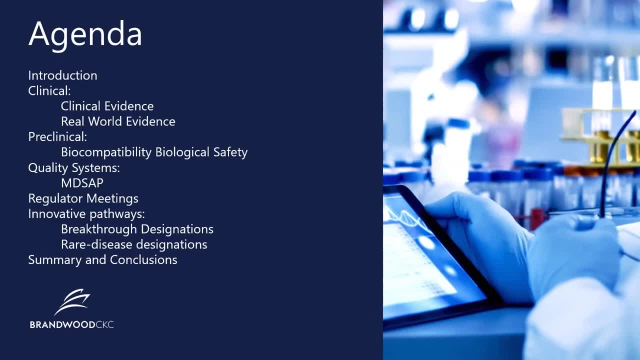 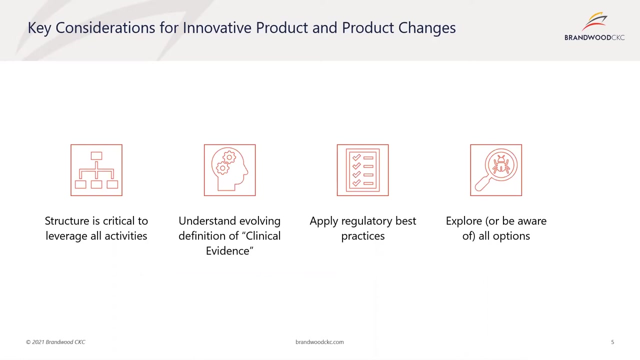 Real-world evidence is a hot word keyword these days. We'll also cover preclinical considerations, quality systems and then regulator meetings, innovative pathways, including breakthrough designations and rare disease designations, and we'll conclude with summary and conclusions, Some key considerations for innovative products and also product changes, As I 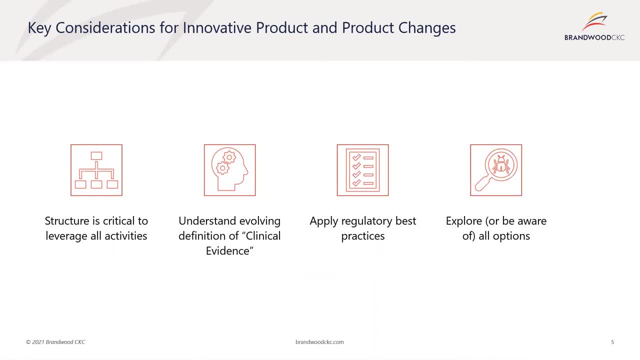 did the research for this presentation and put together thoughts. I thought we'd start with these overarching ideas that really should be encompassing the development of innovative products. First, the structure is critical to leverage all activities. Yes, it's an innovative technology. 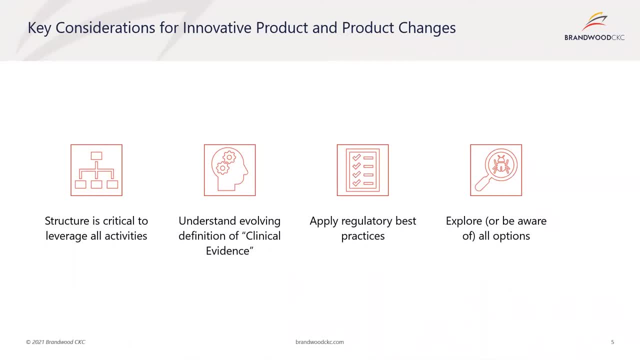 yes, we want to get it to the market as quick as possible. but the more that the development program can be structured and planned, the more the activities can be leveraged from a regulatory standpoint. We want to understand evolving definition of clinical evidence. I'll expand a little bit on that. but 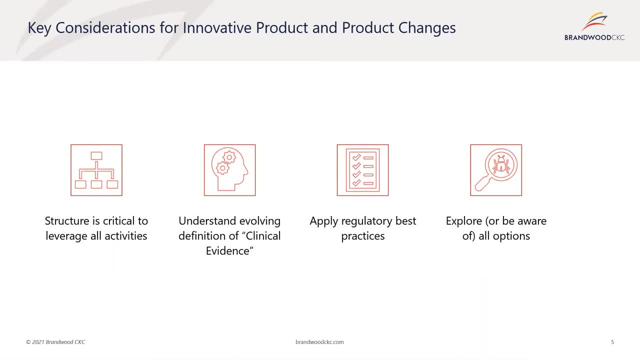 it's not only relying on clinical trials. That definition is ever-evolving, more so these days We'll apply regulatory best practices as a key form from a regulatory perspective. of course, to know what are the current regulatory practices and explore, or at least be aware of, all options would be. 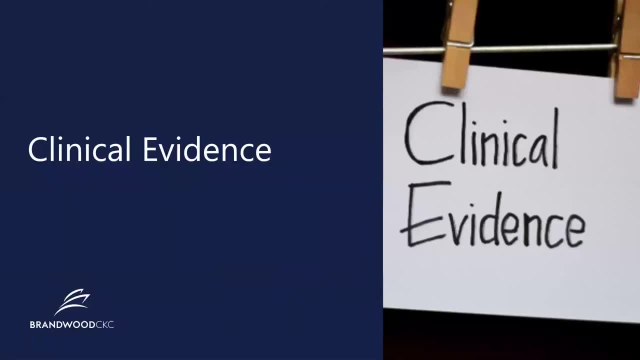 our model. So, jumping into first topic, the first recommendation applying regulatory controls in product innovation is to know the basis very well. Remember, clinical evidence is now globally recognized as all available data, including primary data and secondary data. Waiting to start the clinical evaluation report, the CER, until it is ready to be submitted is a 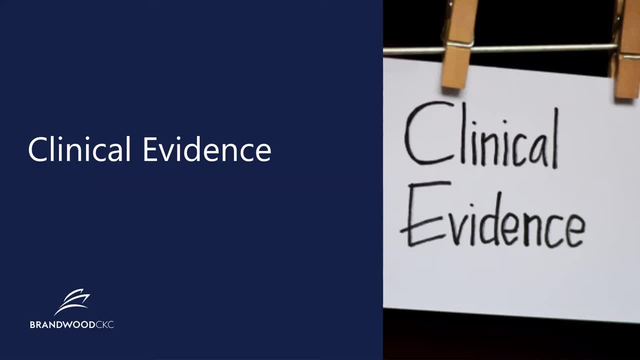 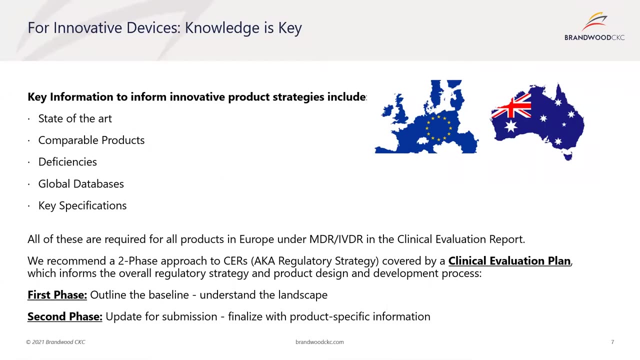 disservice, For example. it would be great to learn what the failure rates and key adverse events are for comparable products as early as possible to learn where to focus on for the new product. So for innovative devices, knowledge is key. That's a model we'll bring to the table. We cannot think of a better way to be. 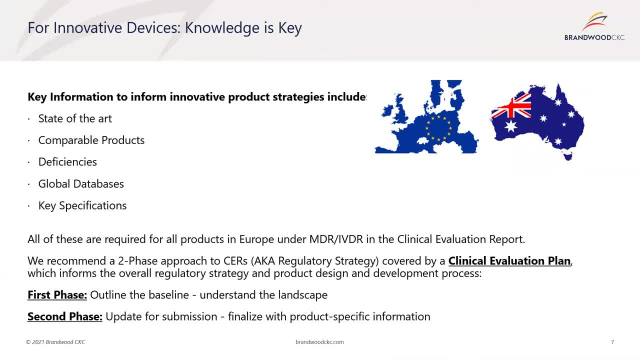 informed than to start with a clearly defined clinical evaluation plan that specifies that at first stage, the CER will be drafted as early as possible. It doesn't have to be formally approved, but it can be maintained and that would be best. throughout the development program, The CER clinical evaluation report are required. 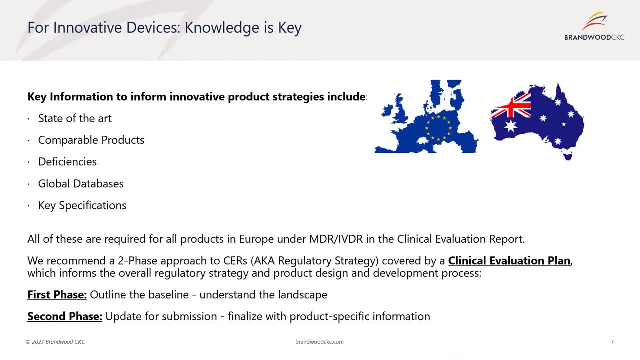 for all device classifications in Europe and Australia. That also applies for IVDs, and the counterpart in IVDs is a performance evaluation report. When primary testing and the product development is complete and is ready for approval, we come back to the CER to run the 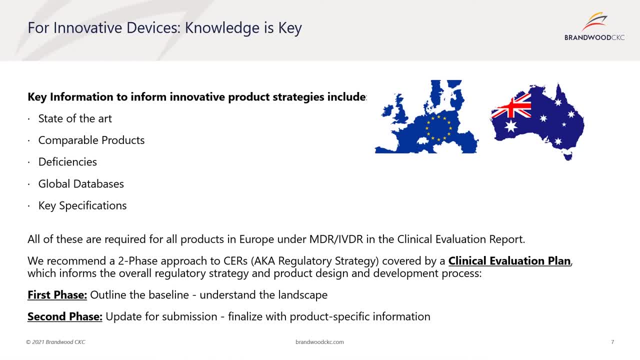 searches and integrate all the information to complete the CER and ready it for submission. Although a CER is not required per se for the US, the information acquired in it will be key for any innovative product, especially as we will outline the analysis on equivalence. 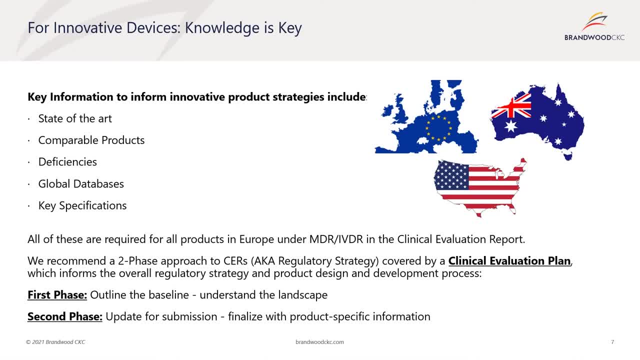 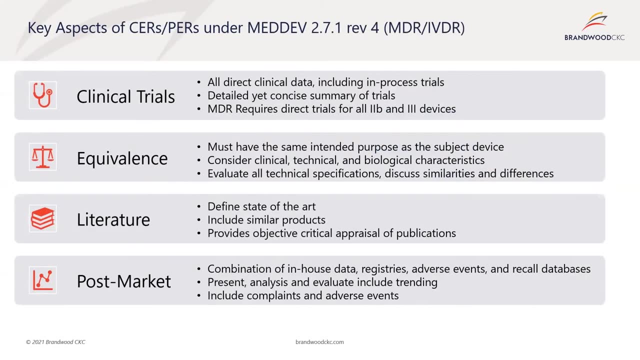 So some of the key areas that are included in the CER is the definition of state of the art, the comparable products deficiency, global databases and key specifications. Jumping a little bit more into detail, There are four key aspects of CERs, which are also key to innovative product development. 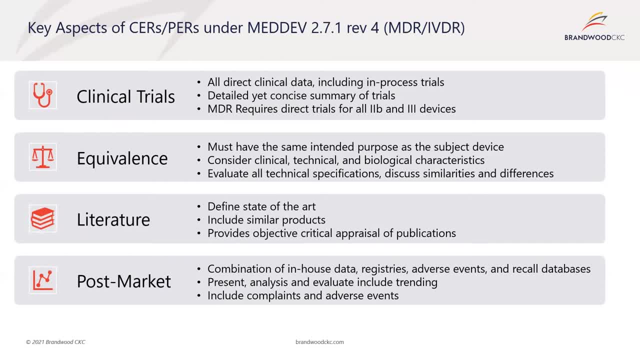 Key aspects of CERs and performance evaluation reports. Under Med Def 2.7.1, Nee 4,, CERs and PRs are required for all classifications on medical devices. They're important considerations, includingricoinclude clinical trials, all basic and recurrent tests. If the devices areios areietet either on Johnson & Günther, NOT be. 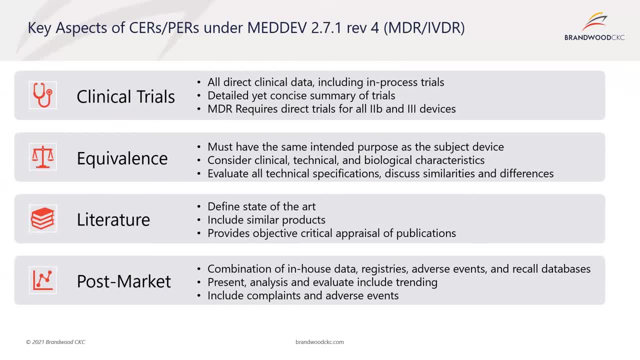 fin, the coroner management or pased-on all china-led Assyrian anesthesia or any choice to their direct clinical data. anything that is in process should be disclosed. the concept of equivalence: it must be the same intended purpose as a subject device if we're gonna claim substantial equivalence but also similar products. 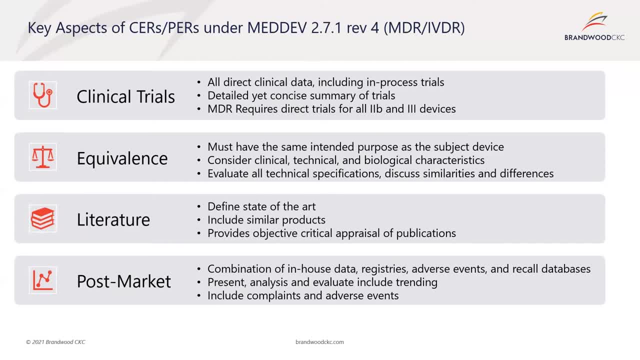 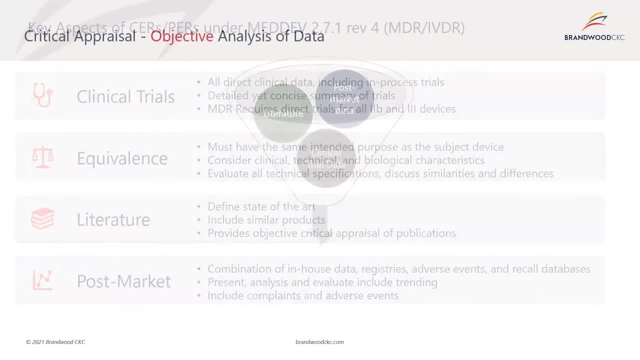 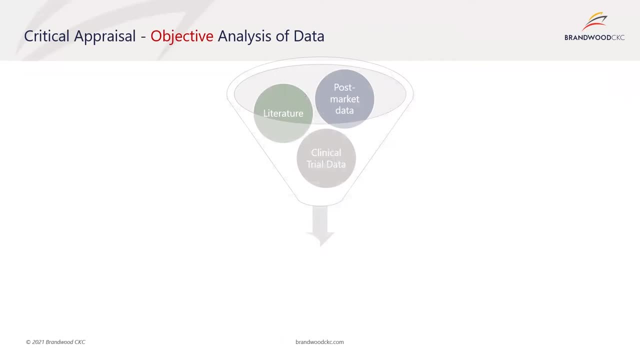 should be evaluated in terms of the literature. we should define the state-of-the-art. it includes similar products and it provides objective critical appraisal publications. the post market is also a critical aspect. so, moving into the critical appraisal, it indicates the objective analysis of the data. we have the literature, we have the post market data, the clinical trial data. 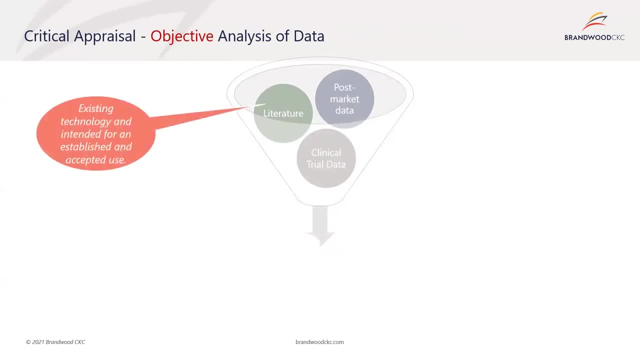 all this is evaluated for both the existing technology and intended for an established and accepted use. new or improving technology. the extension of existing technology to a new clinical use should have direct clinical data and as we move through the next slide, through the critical appraisal, we would generate data on hazards and risks again. 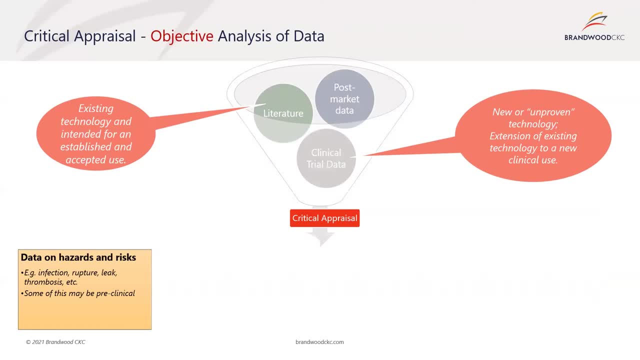 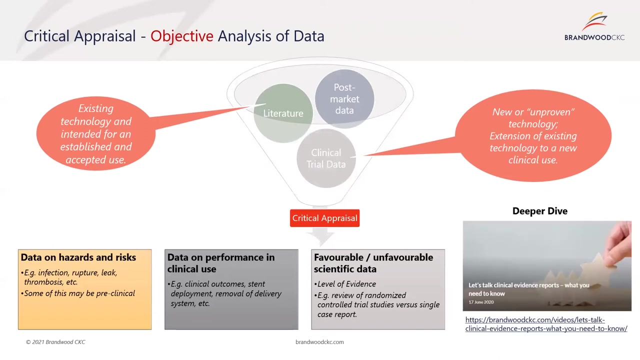 this would be very critical for the development process of any innovative technology. there's data on performance and clinical use. it will generate favorable or unfavorable scientific data and we wanted to emphasize: there is a webinar if we wanted to dive deeper. that really jumps into these topics. so now 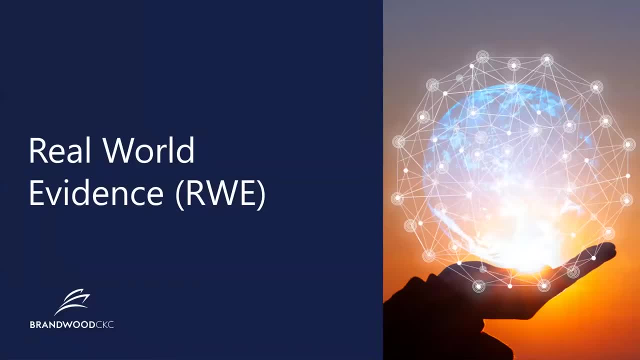 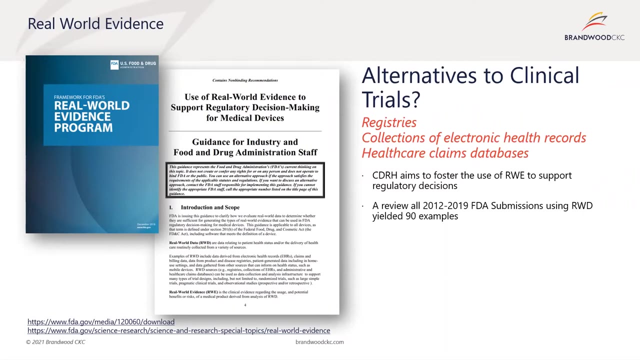 we're going to move to a novel subject: real war evidence. it has been forefront of regulatory innovation, specifically in the US, so we're going to focus on the guidance document for real war evidence and also a very recent report published by the FDA, where it actually provides. 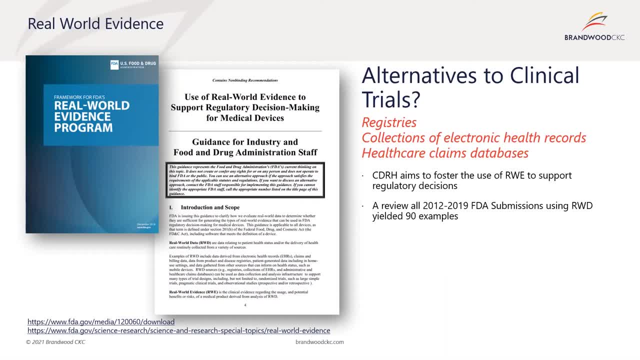 examples of the real war evidence. so the big question is: can real war evidence be alternatives to clinical trials? and the short answer is yes. if we use registries, a collection of electronic health records, healthcare claim databases, this can provide clinical data for registration of innovative Technologies, and we'll jump into some details. a review of all 2012 to 2019 FDA. 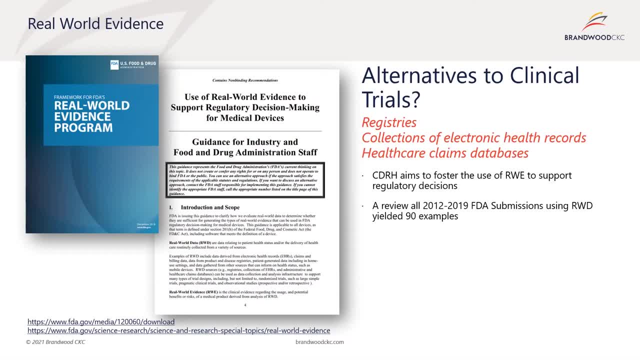 submissions qualified for the use of real war data yielded 90 examples. the report also included examples from areas where innovative device Technologies were being developed. three examples of digital health devices are included, demonstrating the validation of software as a medical device product using real world data, and there's two examples utilizing patient generated data. 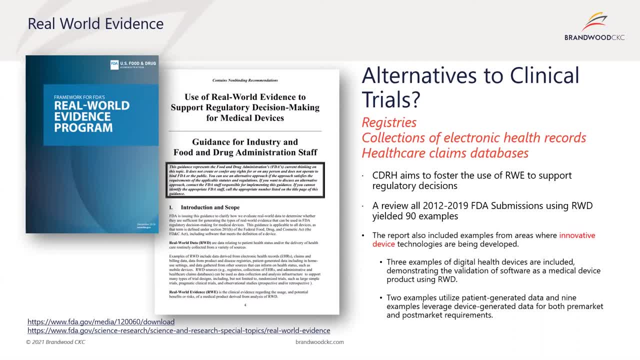 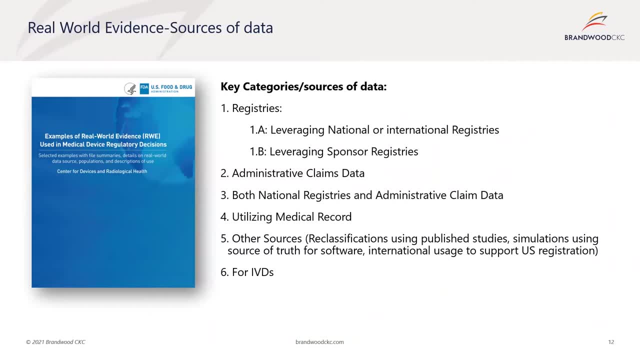 and non-examples. leverage device. generated data for both pre-market and post-market requirements. key categories in the source of data. this is how the report is organized in terms of registries. we see a lot of examples. first, leveraging National or International registries. second, leveraging sponsor registries. administrative claims. 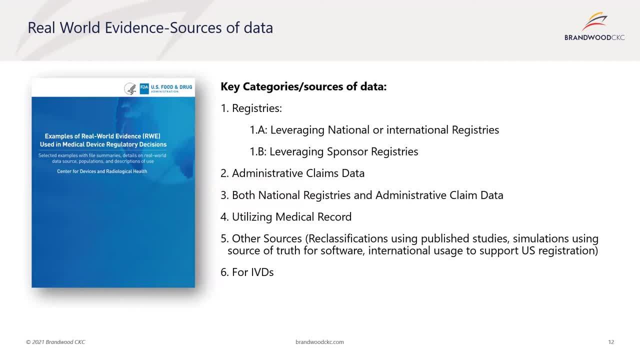 data. it's a second section and, of course, a great source of information as well. the third would be both National registries in administrative claim data and utilizing medical records, other sources, and and then number six was for IVDs. so we said we were going to cover IVDs. 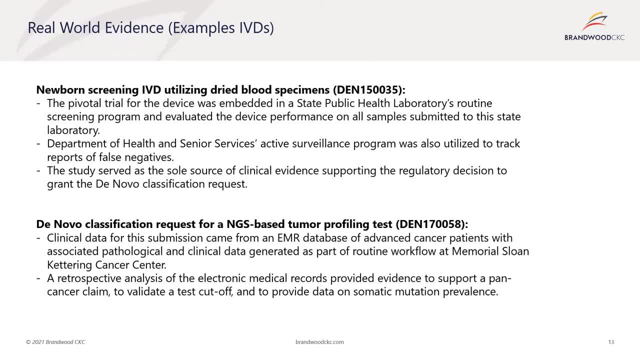 here's an example of real world evidence usage for IVDs. very interestingly, for a newborn screening IVD utilizing dry blood samples, the pivotal trial for the device was embedded in the state public health laboratory routine that was in Missouri the screening program and evaluated the device. 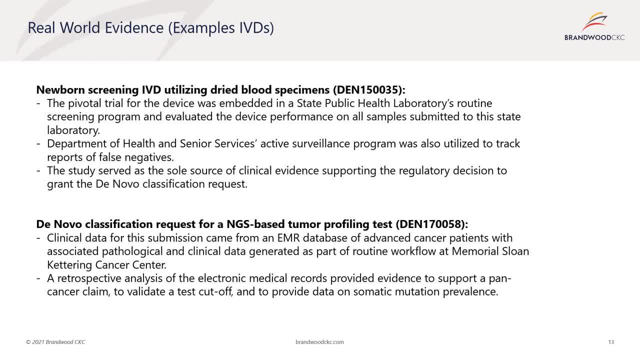 performance on all samples submitted to the state laboratory. the data from this health services office was in the active surveillance program was utilized to track reports for false negatives. the study served as a sole source of clinical evidence supporting the regulatory decision to grant the de novo classification request. I must imagine that must. 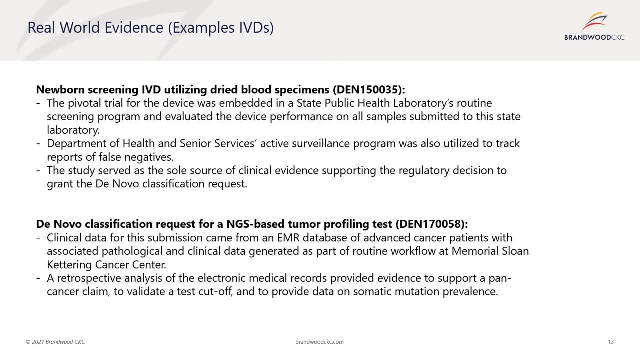 have saved a lot of funding when it was being leverages from a state public laboratory screening database. the second one was the novel classification request from a single generation sequencing based tumor profiling test. clinical data for the submission came from an EMR database of advanced cancer patients at the Memorial Sloan Kettering Cancer Center. a 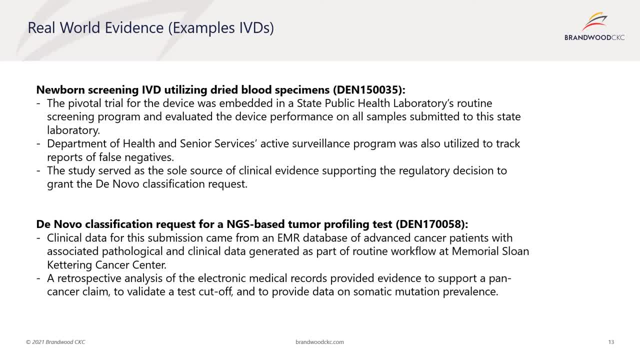 retrospective analysis of the electronic medical records provided evidence to support a pan cancer claim, to validate a test cutoff and to provide data on somatic mutation prevalence. so that was of real-world evidence to validate and to get approval for IVDs. now for product changes. here's: 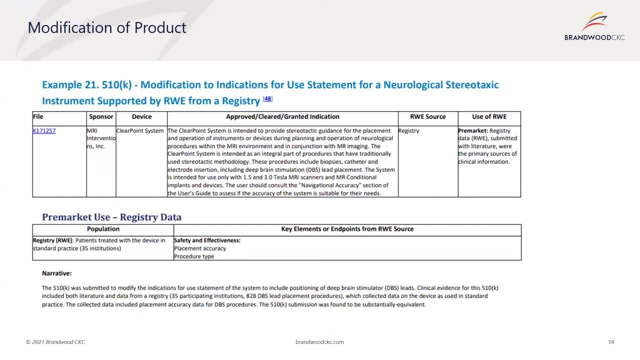 an interesting example. there's a modification to indications for use for a neurological sterile tactic instrument supported by real-world evidence. so you can see in the summary, the 510k was submitted to modify the indications of use, including positioning of deep brain stimulator leads. clinical evidence for this 510k, including both literature and data. 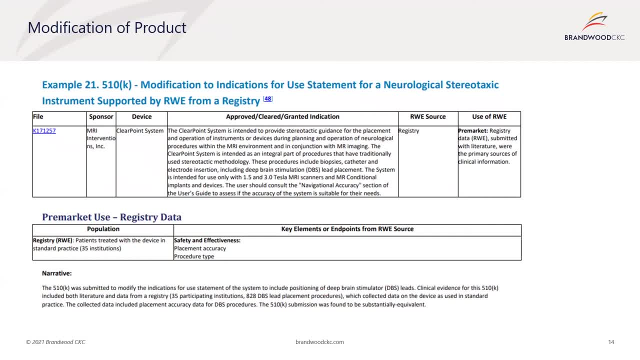 registry, that was, 35 participating institutions, which collected data on the device as used in standard practice, that collected data including placement accuracy for the DBS procedures, and the 510k submission was found to be substantially equivalent. so it's phenomenal: use of real world data and a little bit of foresight really opens the door for leveraging existing data to get an. 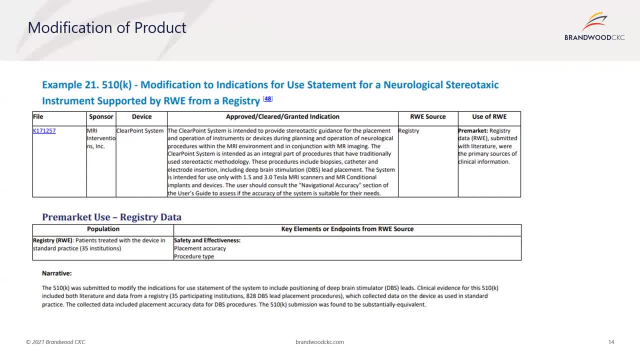 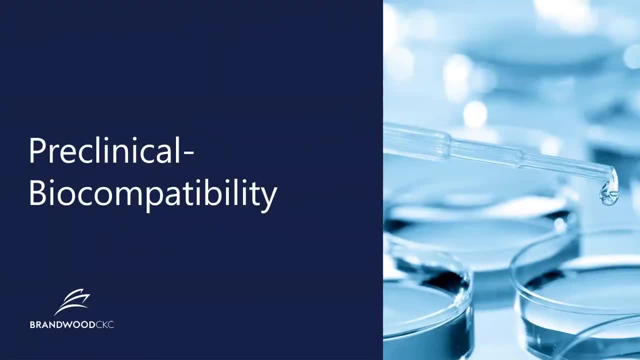 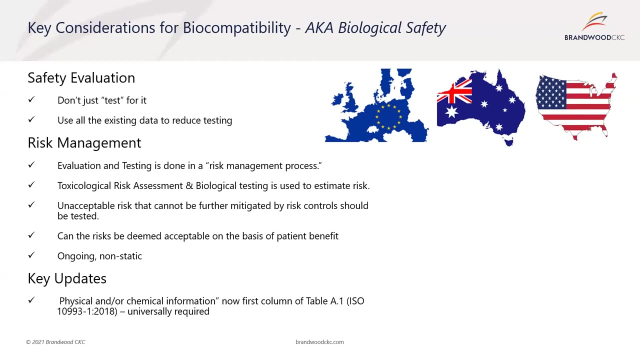 extension of labels, new product registrations in the knowledge. now moving to pre-clinical, we wanted to focus on biocompatibility, biological safety- a very important section- and here's some key considerations for biocompatibility or biological safety, safety evaluation. we just really need to emphasize, don't just test for it, checking the box. 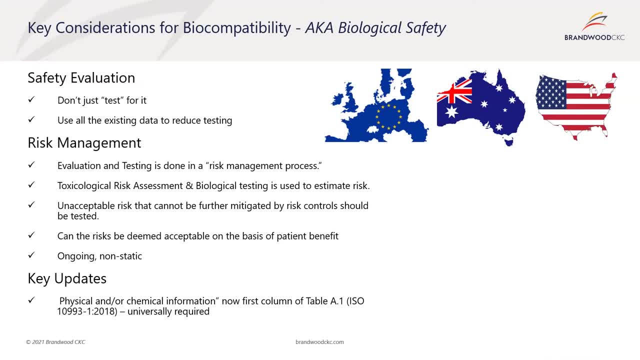 really, in our understanding, hampers Innovation, use all existing data to reduce the testing. so here's where the risk management system really comes into play. evaluation and testing is done on the risk management process. the toxicological risk assessment and biological testing is used to estimate risk. unacceptable risks, that cannot be further. 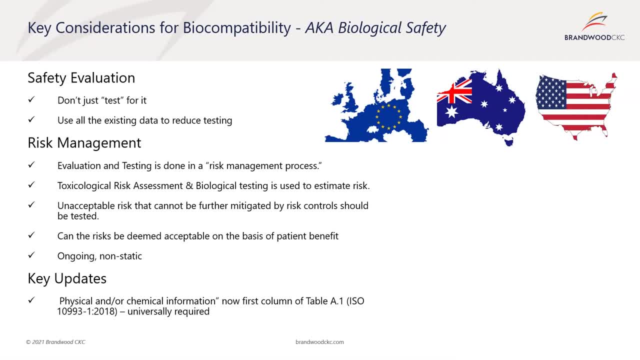 mitigated by risk controls should be tested. this can really answer the questions of: can the risk be deemed acceptable on the basis of the patient benefit and the risk management should ongoing. It should not be static. One important consideration is that physical and or chemical information is now the first column of table A1 in the ISO 10993-2018.. So this is basically. 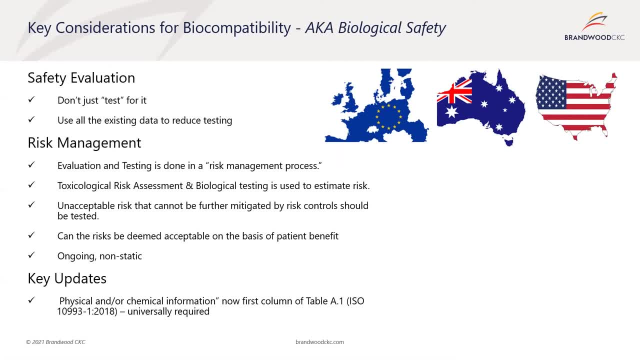 universally required. It doesn't mean that all the testing has to be conducted, but that qualification of the physical and chemical characterization really needs to be addressed for all products. Again, a deeper dive. We've recently- this year- also provided a webinar, So there here's a link if you wanted to jump more in detail into it. So here's how we envision. 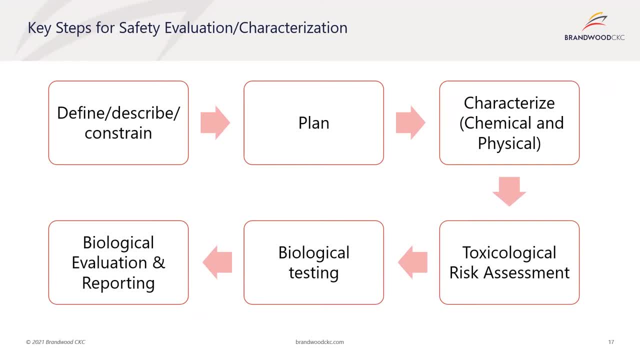 the key steps to safety evaluation and characterization. We want to define and constrain what the type of product is. We would have a plan, We would do that first section, as we mentioned, the characterization, the chemical and physical, and that would lead. 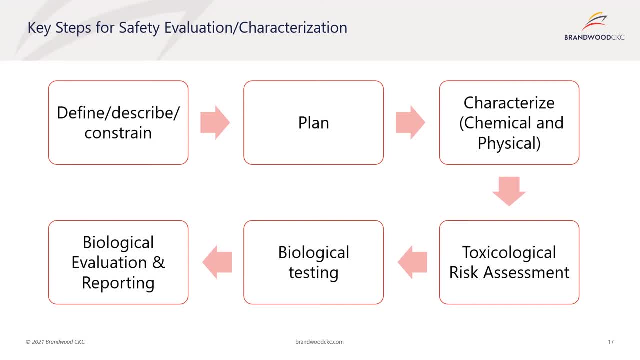 into the toxicological risk assessment, which would identify what additional testing should be done through biological testing. An important thing to do is to start working on biocompatibility at the beginning of the project. It isn't something that you can just slap on the device. 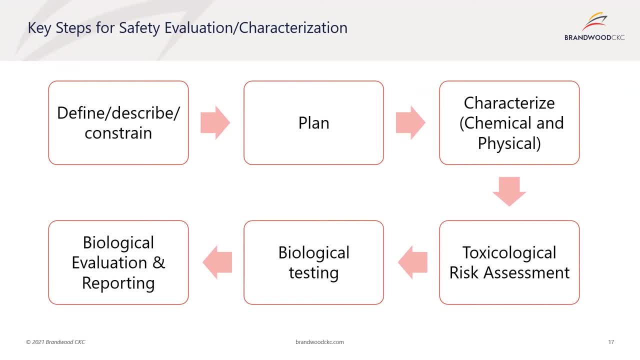 at the end of the project. Even though biological or safety evaluation is a validation activity and has to be done on the final finished product, you should start at the beginning really thinking about this. the toxicological risk assessment and biological testing is used to estimate risk. those risks then. 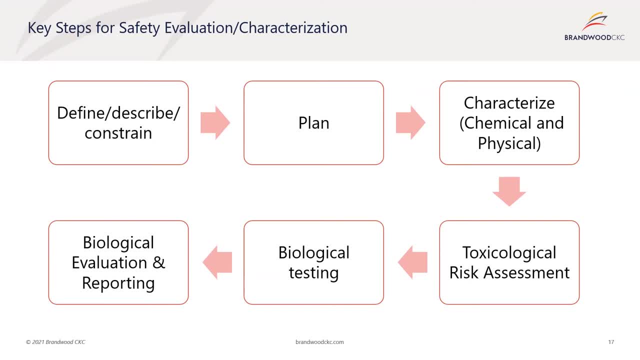 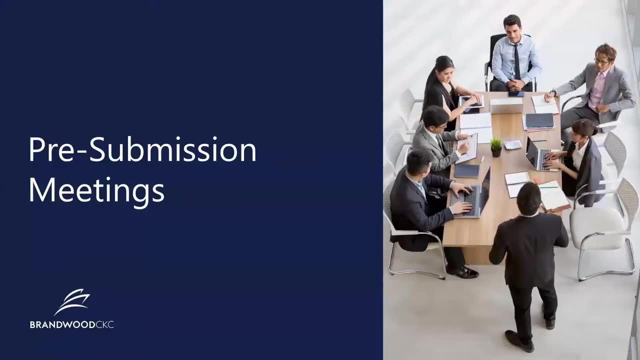 need to be evaluated. are they? are they acceptable or not acceptable? and here's where a multi-faceted, multi-discipline team really comes into play. so now, moving into an important area. there's always that recommendation: going to regulators as early as possible is great, but there's some caveats to 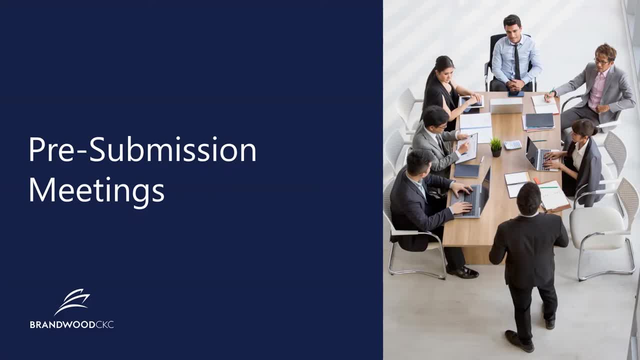 that pre-submission meetings can be valuable tool to reduce risk and ensure that regulators are on board with plans and key decisions. however, as with all things, this needs to be carefully planned and the best practices followed to achieve the best outcome. the worst thing you want to do is 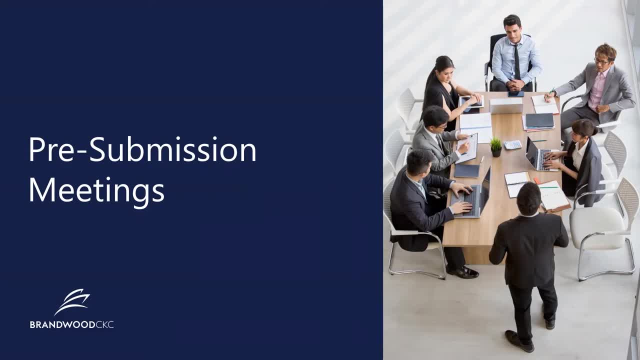 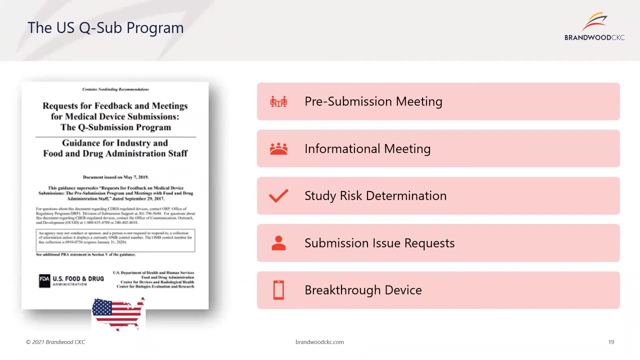 to ask the regulator what he thinks you should do with an open question, the likely answer will be the most conservative option. it's their job to mitigate risk. so let's take a deeper dive on best practices and options. first, we wanted to define uh. we get a lot of questions: um, what is the uh, the pre-submission? 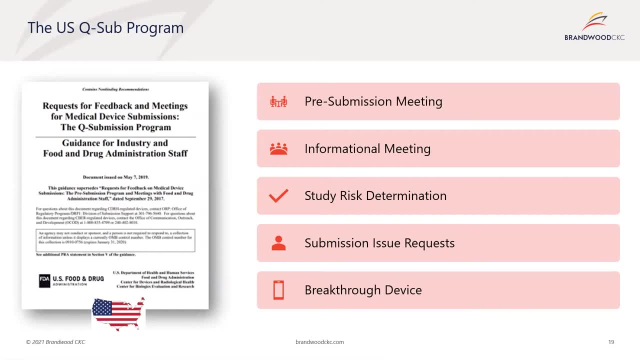 program and all the different jargon with the overarching umbrella for the program. in the us is called the q sub program. we're displaying here, uh, the guidance document. it was originally the pre-ide program in 1995 for id applications. over time the pre-ide program involved to include 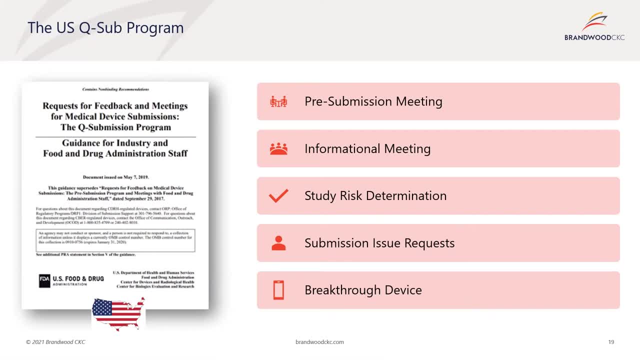 feedback on pmh, the novel request and 510k submissions, and to determine whether a clinical study required submission on ide. well, a lot of things happened and evolved and actually in 2017 the fda defined the q sub program with scheduling and timing of fda feedback for pre-subs. here are outlined the types: 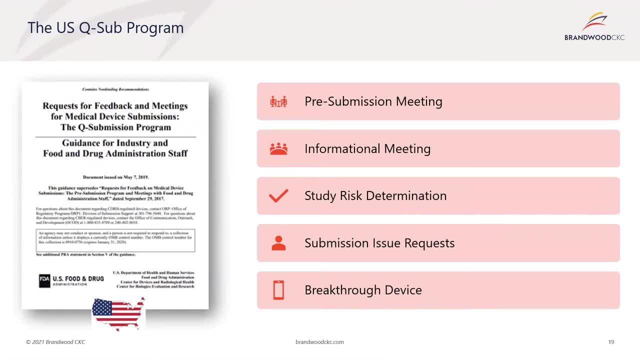 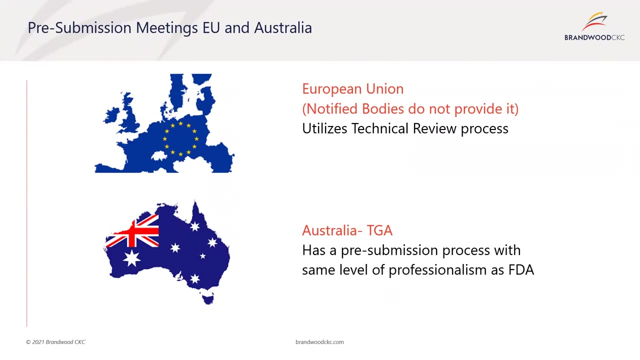 of meetings, the key types of meetings that we have: pre-submission meetings, informational meetings, study, risk determination, submission issue request and breakthrough device application. so now we said we were going to bring a global perspective if we look at european union with mdr and ivdr. even so, more notified bodies will not provide a pre-submission per se or informative. 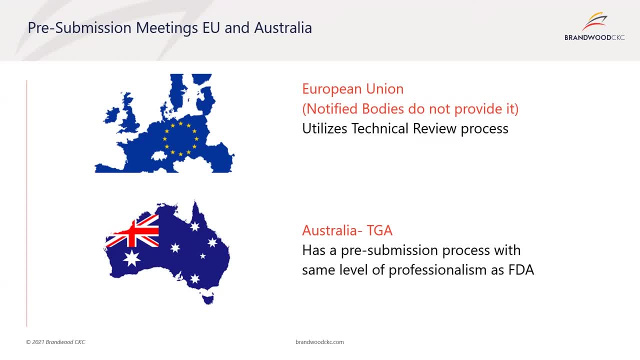 meetings. there is a technical review process. there's some risk because the recommendations tend to be more of a binding nature and they're separate from the notified bodies, so there might be a disconnect there. we want to say the australia and the tga has a pre-submission. 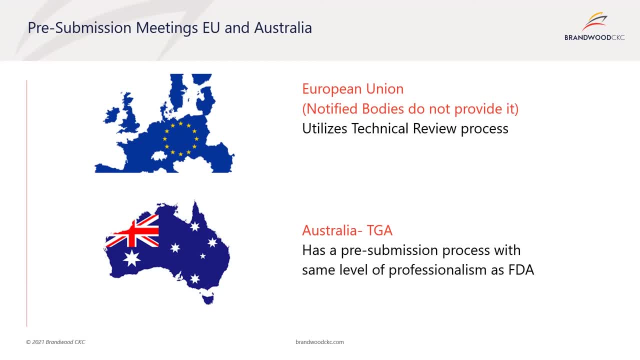 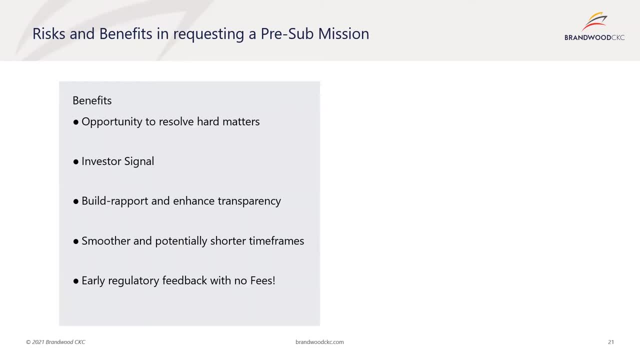 process with the same level of professionalism as the fda. so kudos to that. now jumping into the best practices: we act often with clients do a risk reward benefit analysis. so the benefits of the pre-submission will be opportunities to resolve hard matters. it will show very helpful for investors as a signal to build rapport and enhance transparency. 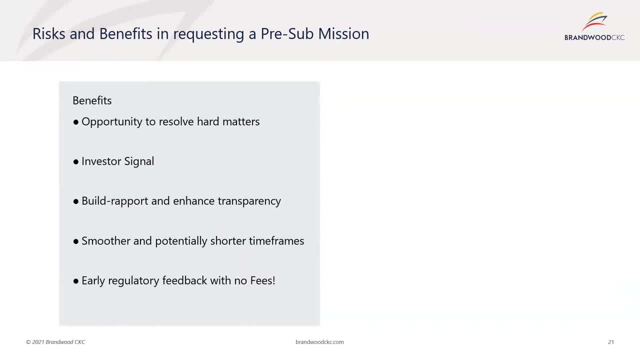 it provides a smoother and potentially shorter time, friends and early regulatory And, generally speaking, both for FDA and for TGA. there are no fees, But here are the risks. First impressions might have implications, So don't make a bad first impression. Don't go so early that you're really not educated. 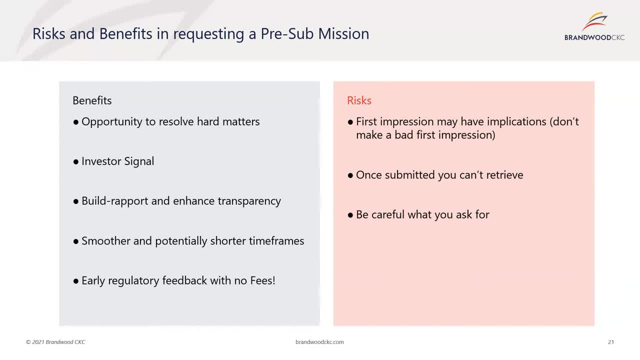 Once submitted, you can't retrieve it, And be careful for what you ask for. We talked about the open-ended questions and that's just really a bad practice to ask: what do you think FDA should do? Should we run a 1,000-patient study? 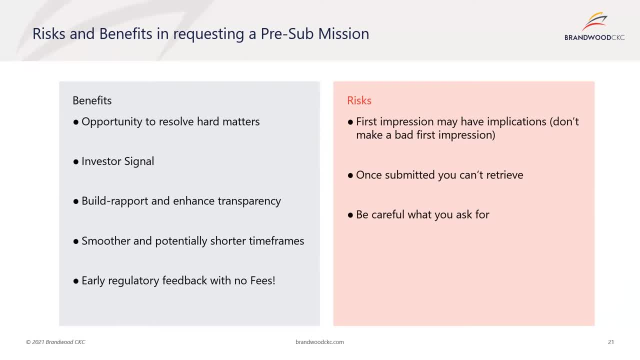 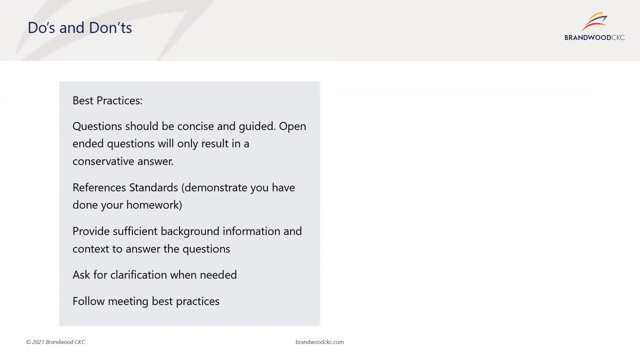 Or use rationale, and usually the answer will be the more conservative one. So, yes, early communication is great, but too early can be a risk. So do's and don'ts and best practices. Questions should be concise and guided. Open-ended questions will only result in a conservative answer. 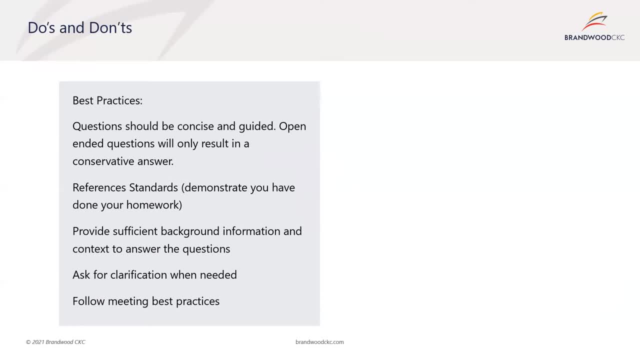 Reference standards as much as you can Demonstrate that you have done your homework. The last thing we want is to be pointed to an obvious reference standard or guidance document where the answers to our questions were clearly delineated, Provide sufficient background, information and context to answer the questions. 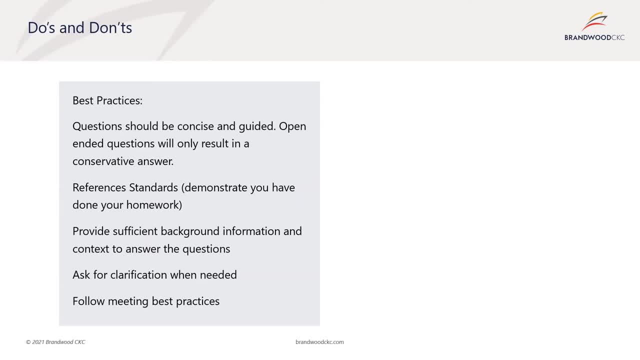 Ask for clarifications when needed and follow best meeting practices. Here's the don'ts. Don't trade a regulator as a consultant. You know it's not their job. The job is to evaluate. Yes, there's some level of advice, but you know it's not their job to answer our questions. 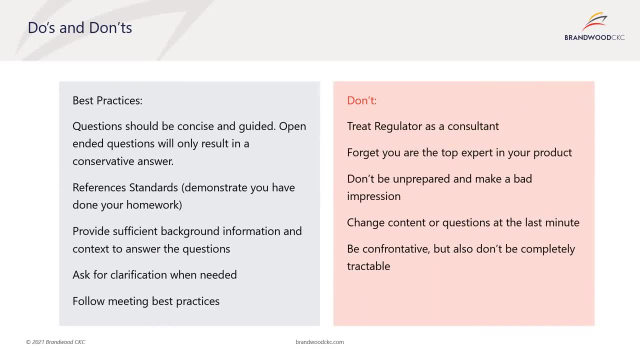 on what we should do for our development. So don't forget that you're the top expert in your product. That's very important. Don't be unprepared to make a bad impression. We named that twice because it's so important. Don't change the content or questions at the last minute. that really will irritate regulators. 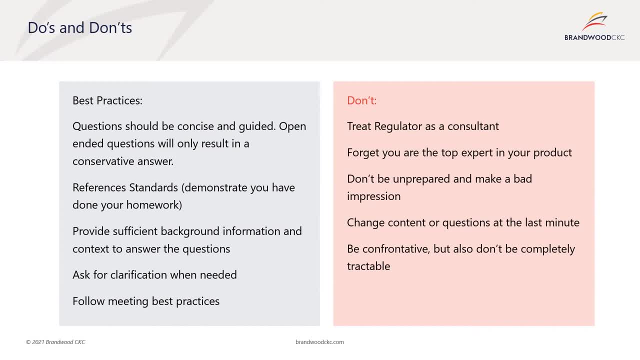 And don't be confrontive, but also don't be completely tractable. You know we're making a negotiation with the regulator, so we want to really make sure we're standing on the sound basis of science, And so there is some room for negotiation. but being confrontative will be a spelling for bad things. 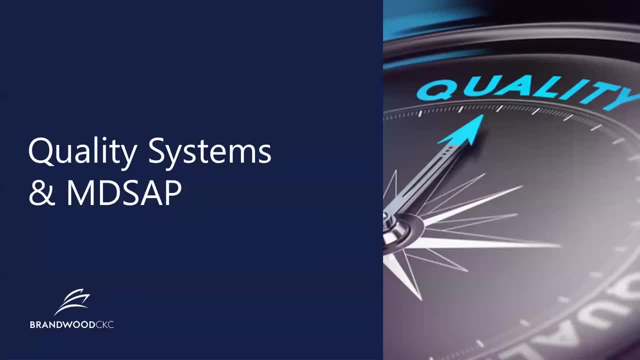 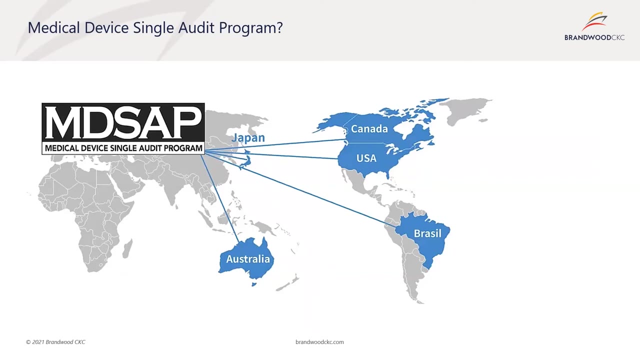 Moving into quality systems and MD-SAP. there can be innovation considerations on the quality system And for us, MD-SAP really encompasses the next stage of how innovative regulatory strategies can be applied to commercialized technologies for product changes. MD-SAP stands for medical device. 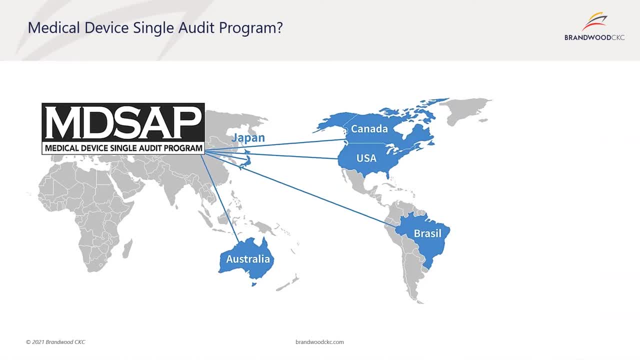 Standardized audit program And I'm just going to name the five key stakeholders and how they use the MD-SAP certification, Starting from Canada. Canada has made it a requirement, So any early innovator who's thinking of commercializing a product globally and includes that, includes Canada. 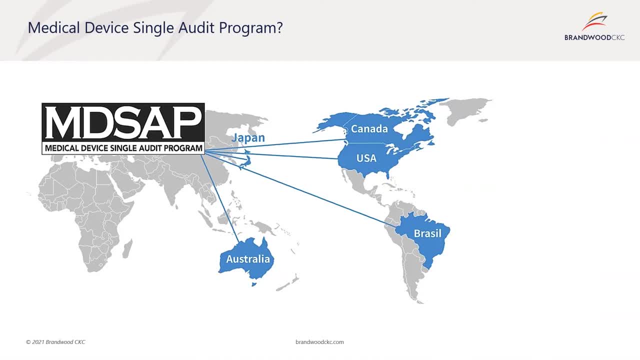 there is a requirement for quality system certification. The US recognizes MD-SAP, one of the key stakeholders. Anvisa will also recognize in Brazil the MD-SAP certification. Japan uses this as also manufacturing evidence And, interestingly, Australia now uses MD-SAP for registration purposes. 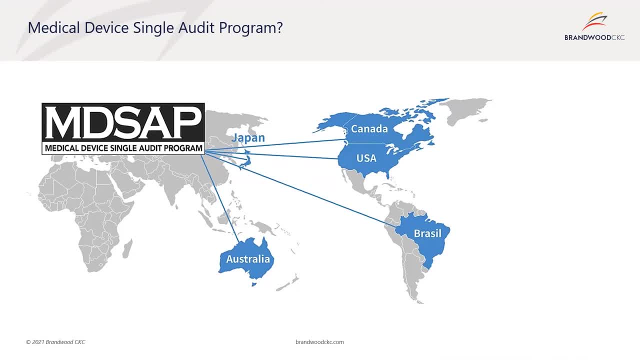 So whereas before Australia would only recognize a 13485 and CE mark, now MD-SAP certification plus a 510K or Japanese or a Canadian certification is a requirement. So any early innovator who's thinking of commercializing a product globally- and includes that, includes Canada- there is a requirement. 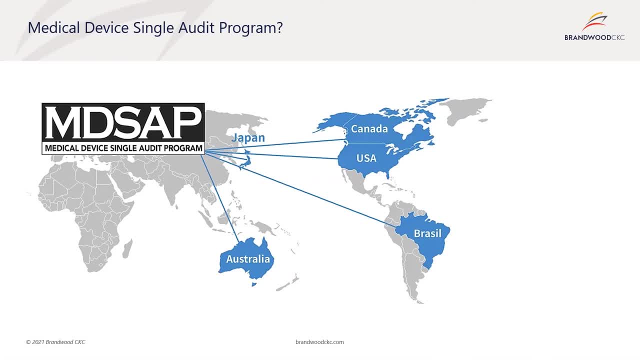 So for Canadian approval, so long as the same product risk category is observed generally, can be used to register new novel products in Australia. I also wanted to mention the World Health Organization, WHO is an observer, and the SAP, and that the European Union are official observers as well. 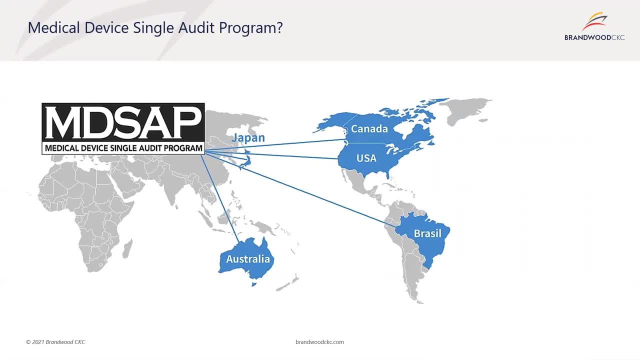 So at some point- maybe after they're done- with MD-SAP certification when you make an order. So any early innovator who's thinking of commercializing a product globally and includes that, includes Canada. there is a requirement. So any early innovator who's thinking of commercializing a product globally and includes that, includes Canada. there is a requirement. 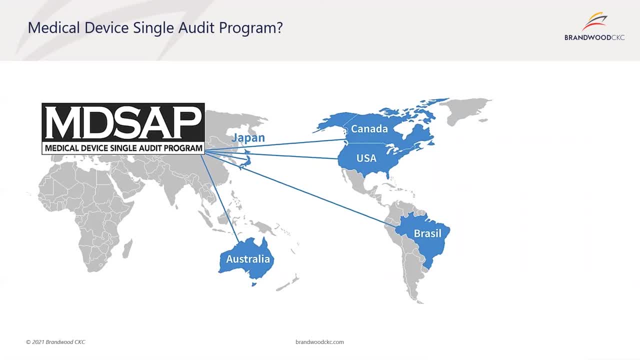 So any early innovator who's thinking of commercializing a product globally and includes that, includes Canada, there is a requirement and IVDR and Brexit- they might be recognized as MDSAP as well. If you want a deeper dive, and then what MDSAP? what that entails. here's also a link that we did this year, recently And let's jump. 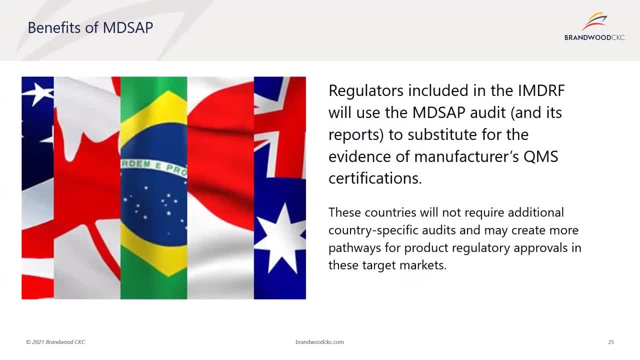 into the benefits of MDSAPs. Regulators included in the MDRF will use MDSAP audit and its reports to substitute for the evidence of manufacturer's QMS certifications. These countries will not require additional country-specific audits and may create more pathways for product regulatory. 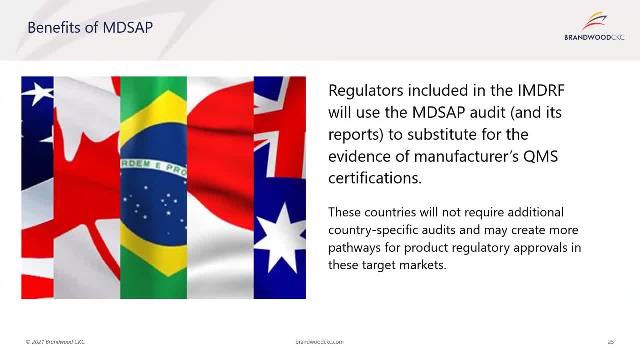 approvals in these target markets. So the regulators reserve the right to still do a forecast audit, but essentially by signing into the MDSAP voluntary program. if there's not a forecast audit requirement- for example FDA, Canada or Japan- they will not come and do a. 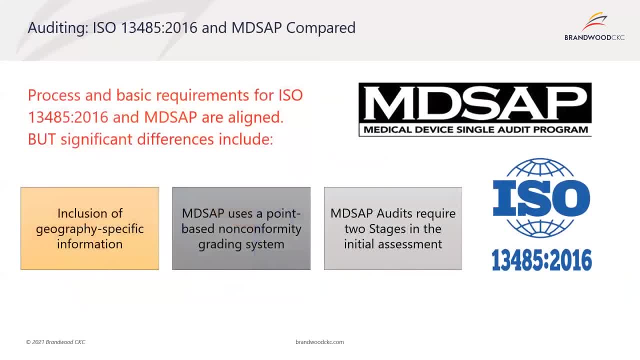 surveillance audit. That's, generally speaking, the benefit for MDSAP. The process and basic requirements for ISO 1345 and MDSAP are basically aligned, but there's some significant differences. This includes inclusion of geography-specific information. It also includes a point-based non-conformity grading system that has to be 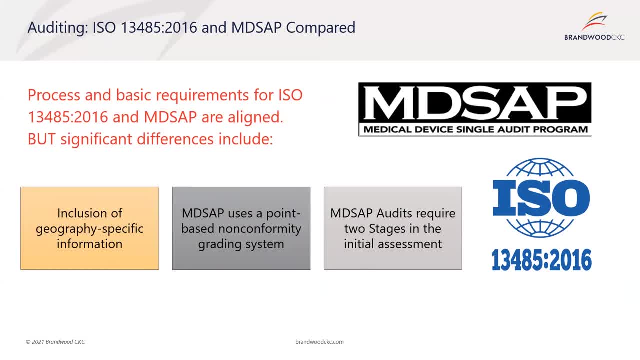 very carefully observed. The MDSAP audit requires two stages in the initial assessment. however, from an innovative regulatory strategy standpoint, how we envision it is that really the gap between ISO 1345 and MDSAP is about 20%, And if we ask the notified body to do the certification, 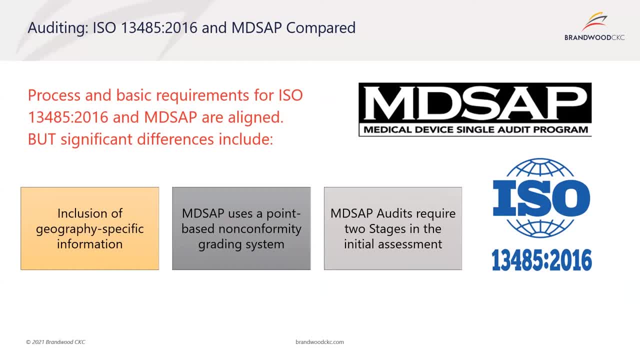 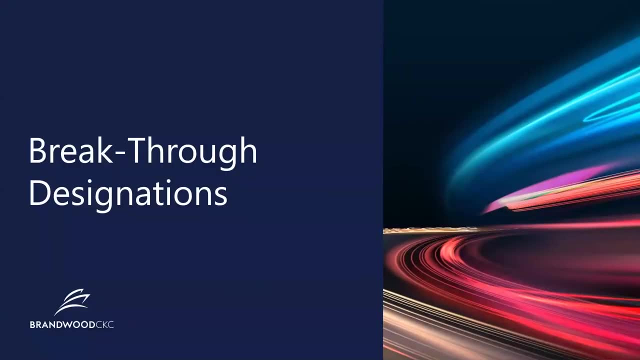 audits for both, it really doesn't create a significant additional hurdle in the amount of work. So that's sort of something to think about early on and we believe it's a very good example of innovative strategic thinking. Now jumping into details for more classical 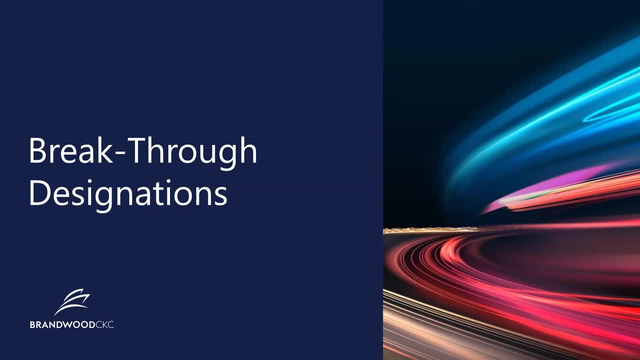 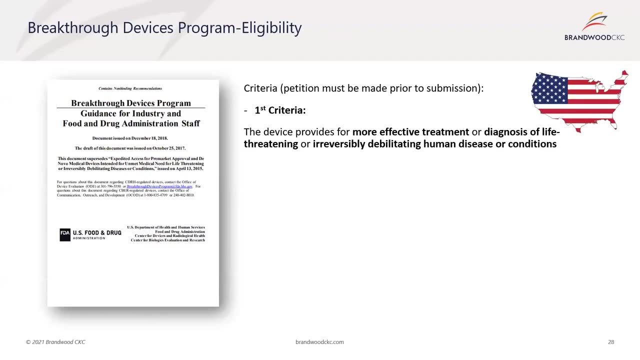 considerations when we're talking about innovative products. let's talk about breakthrough designations. Breakthrough designations are something that is really exciting for innovators. Let's talk about the criteria for the US. The first criteria really constitutes the device that is designed to be able to provide a more effective treatment or diagnosis of life-threatening. 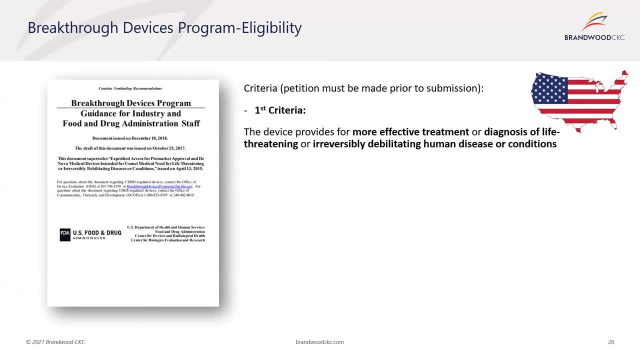 or irreversibly debilitating human diseases or conditions. That has to be documented in the application for a breakthrough device. Secondly, one of the following needs to be met: The device represents breakthrough technology. No approved or cleared alternative exists. The device offers significant advantages over existing cleared or cleared alternatives. 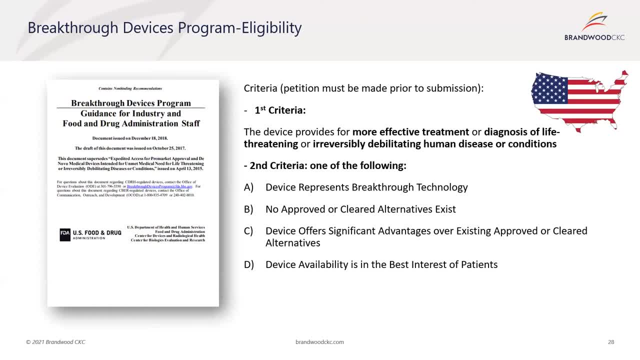 Availability is in the best interest of patients. Now a couple of caveats. Multiple devices with the same intended use can be issued breakthrough designations, but only one. the first one will be approved. Once that first product is approved, the FDA has reserved the right to not. 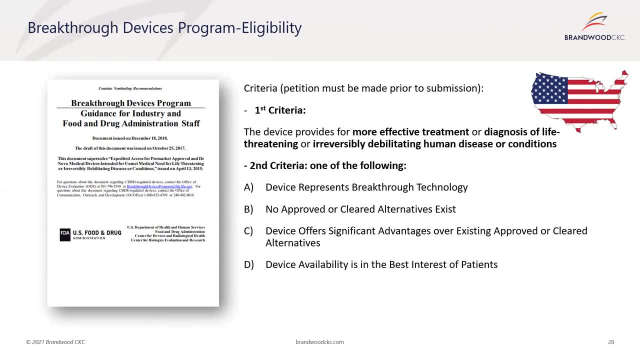 continue to issue breakthrough designations, probably because the device would no longer represent a disease. Now the first product is approved, The FDA has reserved the right to not continue to issue breakthrough designations, probably because the device would no longer represent a disease. 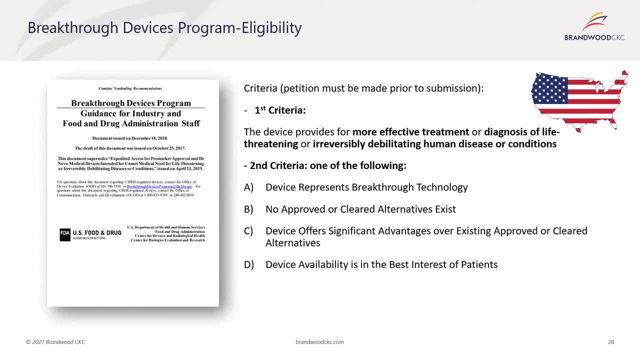 Direct breakthrough. Now there could be multiple products for the same indication- disease- but not with the same indication. I also wanted to mention that the breakthrough device program superseded the expedited access pathway and the innovation pathway. Here are the benefits of getting a. 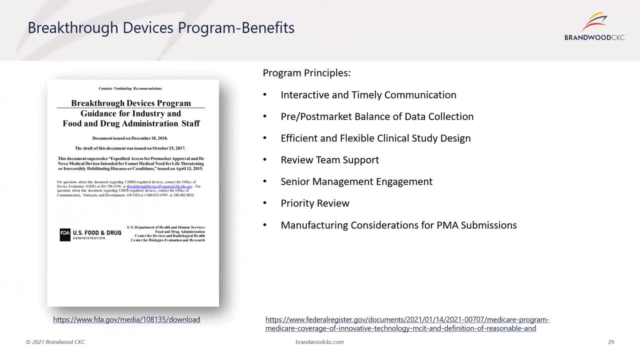 breakthrough device. The submission program now becomes interactive and FDA is pressured to provide more timely communication. There will be pre and post market balance on data collection. Efficient and flexible clinical study design can be applied inren aup gegenüber recommended. Here is one of the few examples where the FDA would really collaborate to identify. 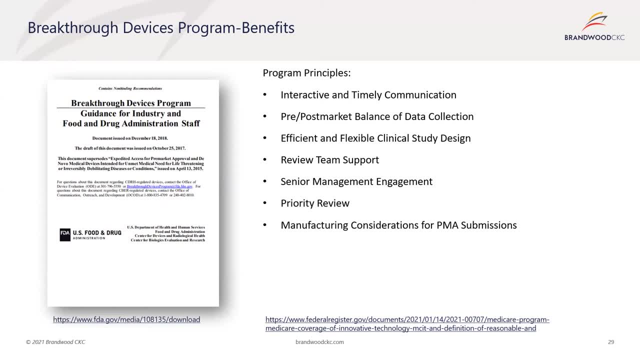 what would be the most efficient way to get the product registered. There will be review team support. Senior management will be격ted with the criteria but not with the gnome to either follow or perform GTmC0t effect. There will be review team support. senior management will be engaged from the FDA standpoint. 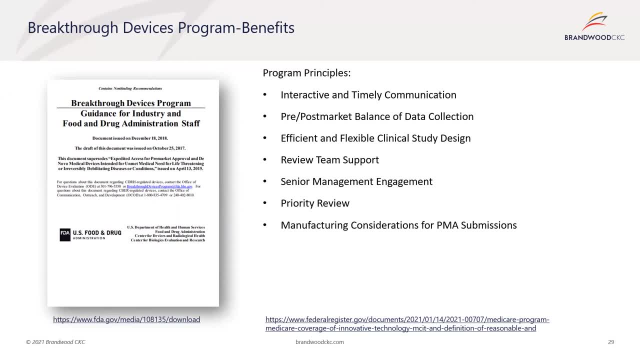 The submission comes a priority in terms of review so that there is a shortened timeframe in their manufacturing considerations from PMA submissions. An additional benefit, which unfortunately is now on hold, is that the Medicare coverage of innovative technologies, the MCIT, as of January of 2021, had approved instantaneous 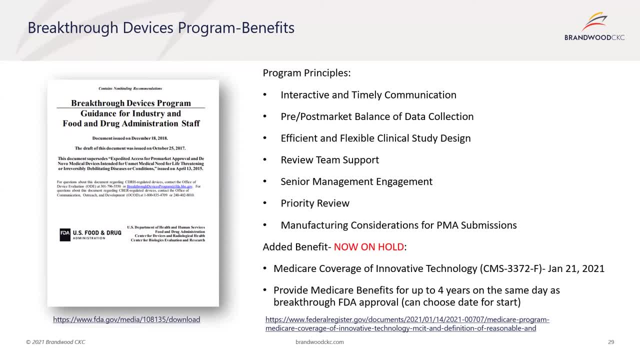 coverage for Medicare for any product that got approved by FDA through the Breakthrough Device Program. Unfortunately, the program is currently on hold. There's an open consultation that is evaluating how the coverage could be determined and what kind of controls, So it seems like the 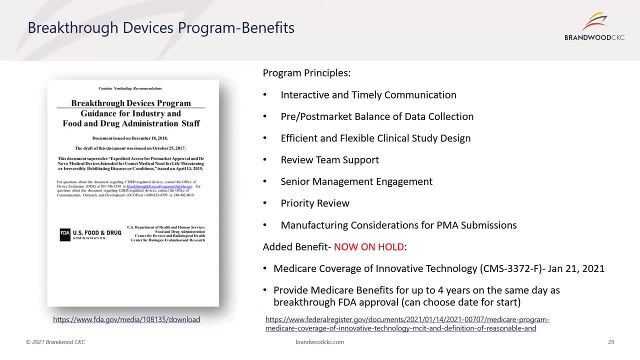 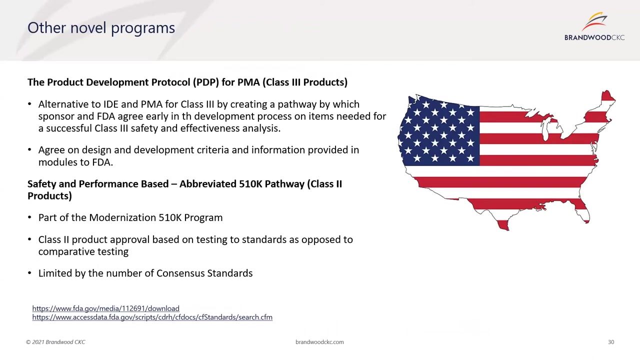 The benefit kind of got a little bit ahead of the curve and now they're pulling back. but our hopes is that that will be reinstated, because it really provides a tremendous opportunity for getting innovative technologies covered instead of that reimbursement process being so lengthy. There's other novel programs worth mentioning from FDA. 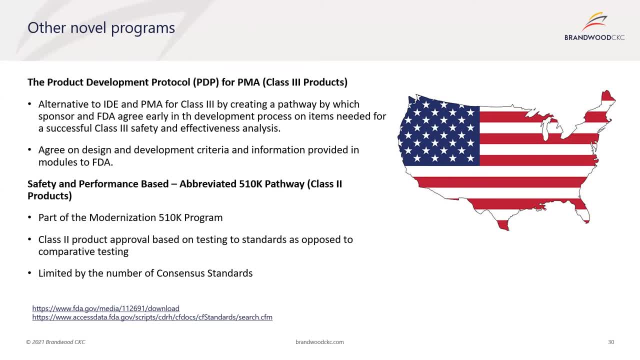 Of course there's quite a number of them, but here's two that I particularly want to mention. The product development protocol, the PDP, is applicable to PMAs class three products in the US. Essentially the FDA will agree on the product development plan and if that protocol is followed, 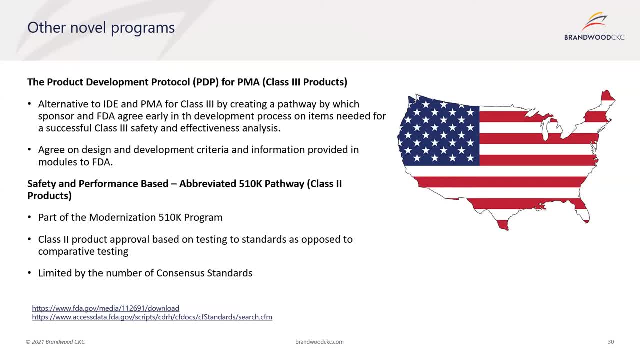 then basically that is sort of providing the game plan for approval. The FDA will agree on the design and development criteria, and the information is provided in modules to FDA, And so there could be more interactive feedback. There's another one called the safety and performance-based abbreviated 510 pathway. 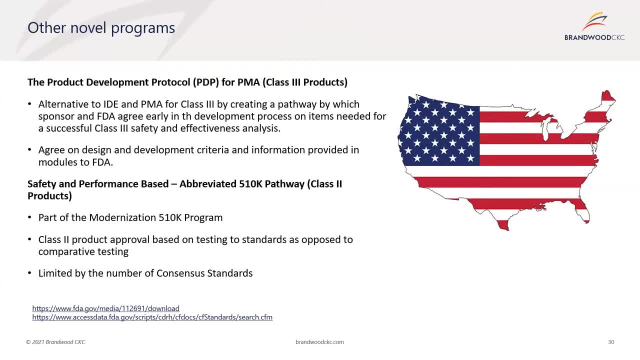 This is for class two products. It's part of the modernization 510 program. It applies for product approval based on testing standards as opposed to comparative testing. Remember that 510 is approval pathway only for substantial equivalents, And so that's why we've been working on this. 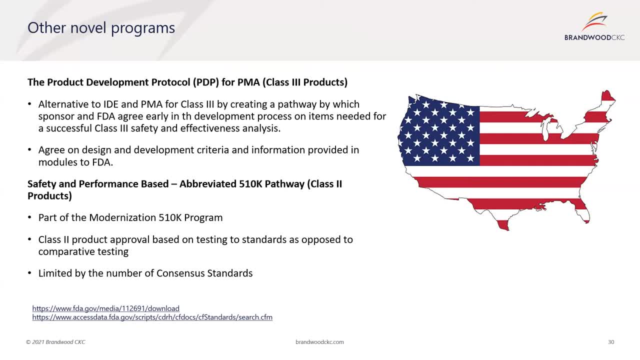 So that's why we've been working on this, All right. So it just kind of goes back to some of the concerns I had when we were trying to get artificial intelligence or artificial intelligence test to approve a product. So with this new process you can get a product approved without substantial equivalents based. 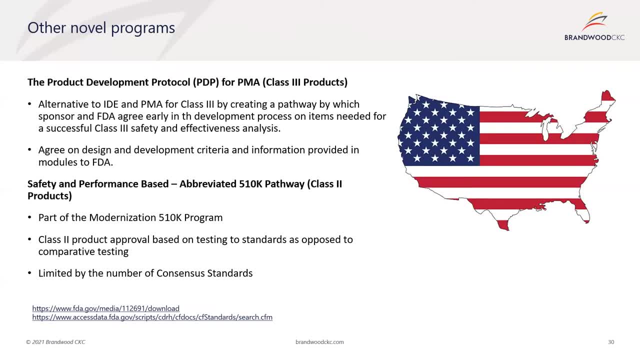 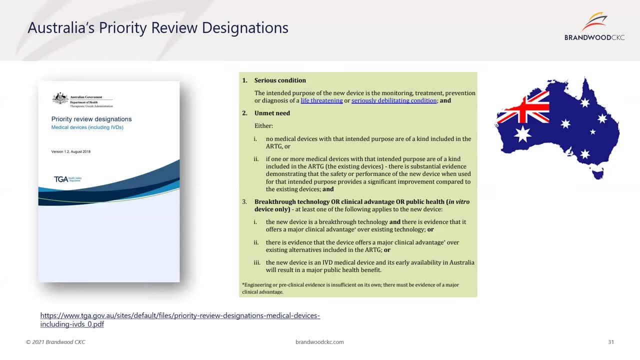 on consensus standard. However, there is a limited number of product-specific consensus standards, So the program is intended to continue to grow in the near future. Now moving into Australia's Priority Review designation: Australia does have a Priority Review designation. It is modeled after the US. 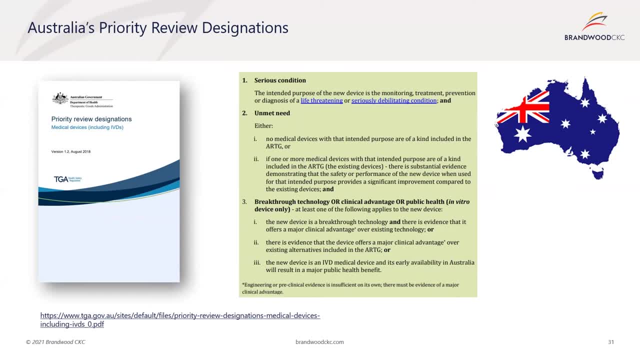 So they have the Commission of Prospects, which has the short-term rating in the past 30 years. um, i was reading the consultation document when they were considering how to structure this. really, the benefit is it provides the top of the queue, so it's intended to be a faster approval. 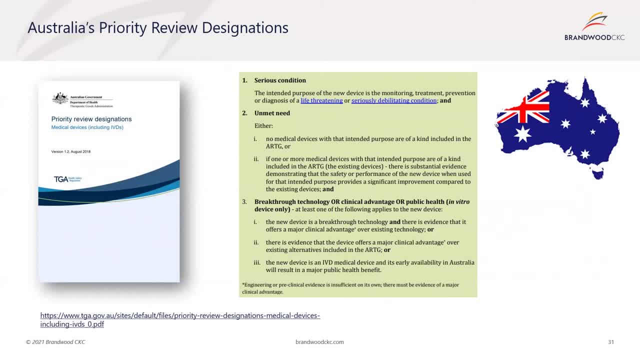 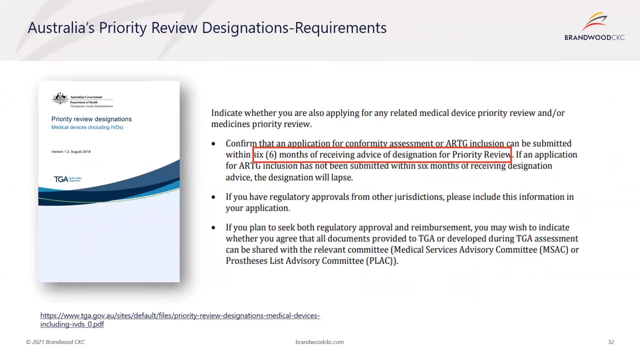 here are the conditions, again very similar to the us. there's a serious condition, unmet need and breakthrough technology, or clinical value advantage or public health benefit. however, it really should be used, uh, very differently than the fda's approval process. here's why, for a priority review designation, there is an expectation that the full application will be. 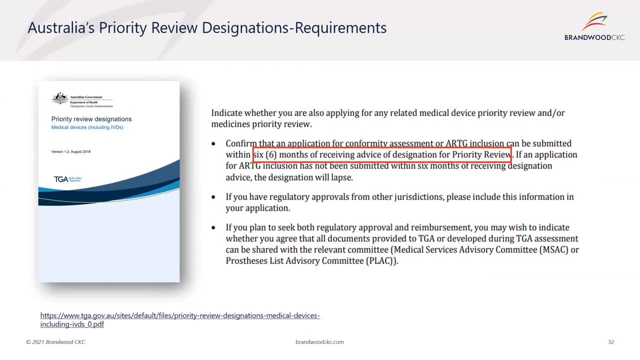 submitted six months after receiving the priority review designation. so that really means that companies need to make this application when they're ready to submit the full documentation for the application. It can't be six months. longer than six months. There is a way to renew the prior review designation, but it's not the best, not advisable. 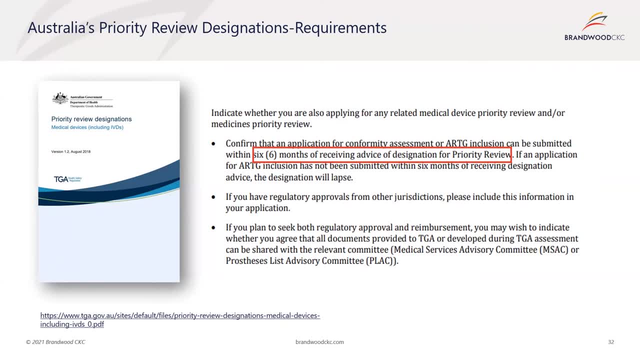 So I did want to mention there is a fee for this prior review application of about $9,000 Australian dollars since 2018. as of today, The designation decisions. unlike the US, they will be published on the TGA website after you have been notified. 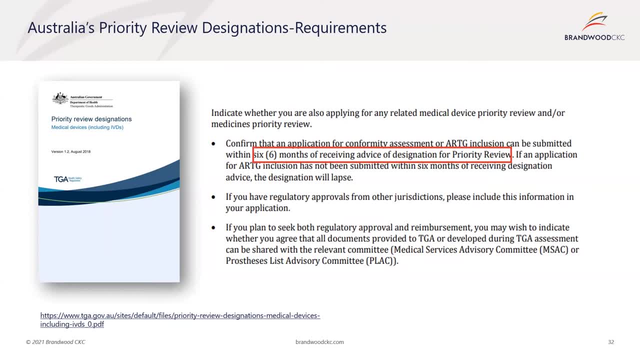 Applications with a granted prior review designation will be allocated front of queue priority throughout the relevant assessment process. This includes TGA's business processes associated with the applications for conforming assessment and inclusion in the ARTG for medical devices. So what's happening in Europe? 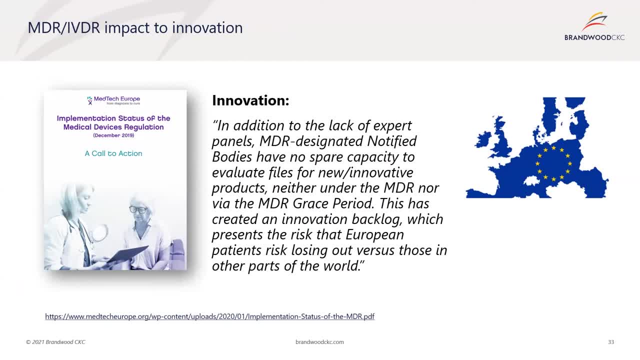 I thought it'd be Best narrated here by MedTech Europe. MedTech Europe is the European trade association for medical technology and industry, including medical devices, diagnostics and the such. MedTech Europe's mission is to make innovative medical technologies available to more people. 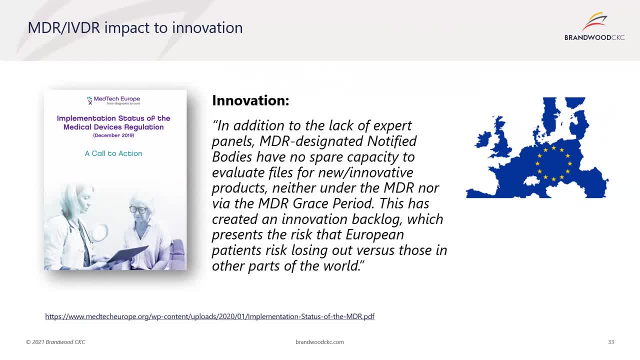 Here's the conclusion: 2019.. In addition to the lack of expert panels, MDR designated notified bodies have no spare capacity to evaluate files for new innovative products, Neither under the MDR nor via the grace period. It has created an innovation backlog which presents the risk that European patients risk losing out versus those in other parts of the world. 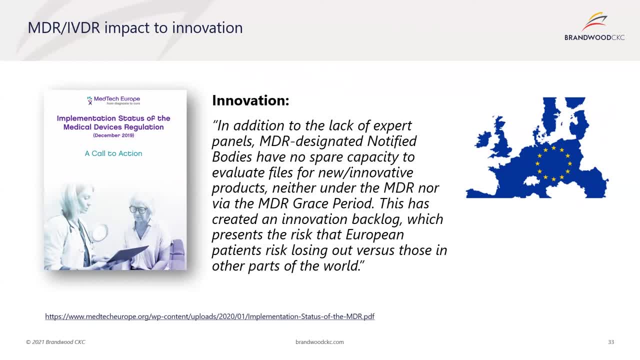 So unfortunately, the impact of MDR and IVDR does not look the most positive to innovative technologies, But nonetheless we're working with companies that have managed to overcome these hurdles and are certainly way in the way to meeting MDR certification or IVDR. 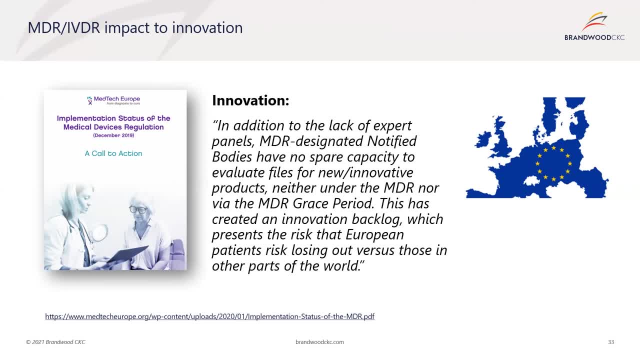 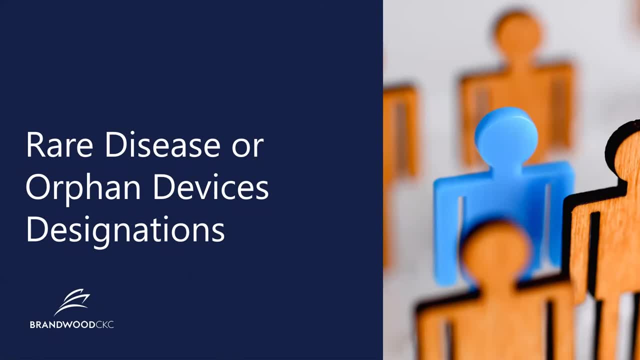 And so it's not universal, but certainly an impediment at the moment. An innovative path which cannot be complete in terms of an analysis without touching on rare diseases or orphan device designations. This program, against spearhead by the US, really offers some very unique advantages for innovative technologies. 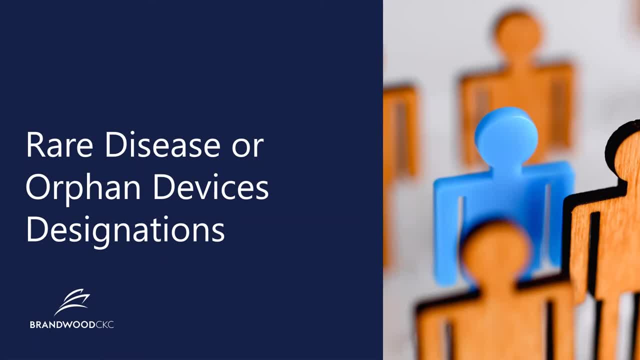 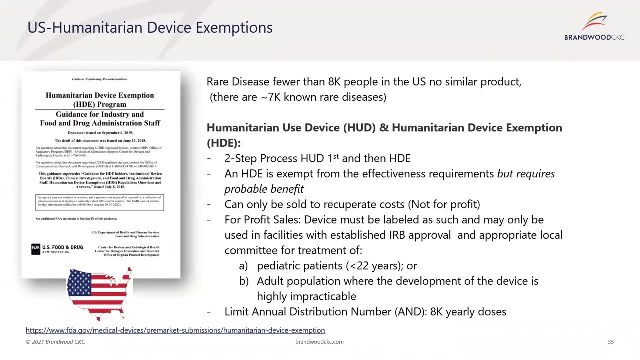 Even those that are not particularly Solely applicable to rare diseases or solely developed for rare diseases. Here's a little bit about that. So in the US the humanitarian device exemptions, the HDE, is the approval for rare disease indicated medical devices or diagnostic products. 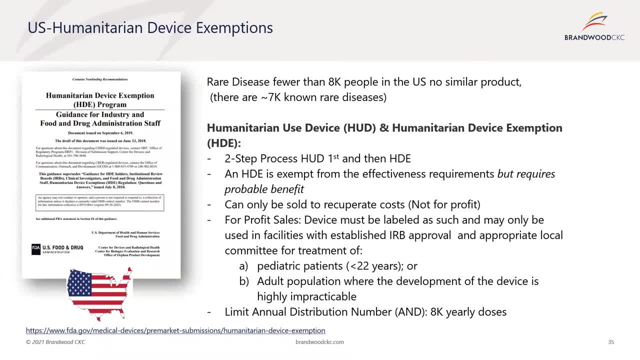 It's a two step process. First the HUD humanitarian use device needs to be issued, and then the HDE, A rare disease, is defined by each country According to our population, but in the US, as of most recently, it means that no more than 8000 people are affected in the US. 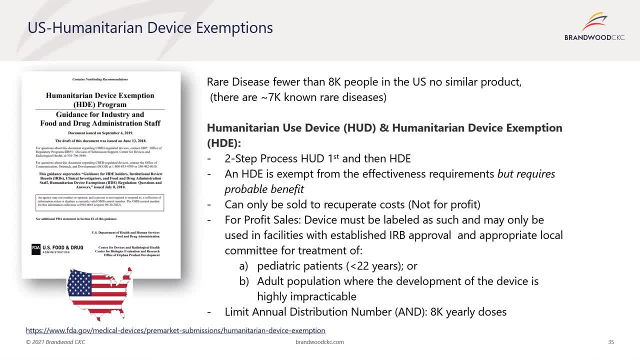 There's a requirement that there's no similar product And I wanted to mention there's about 7000 known rare diseases. An HDE is exempt from the effectiveness requirements but requires probable benefit. What that means is that By default, these products are PMA class three products. 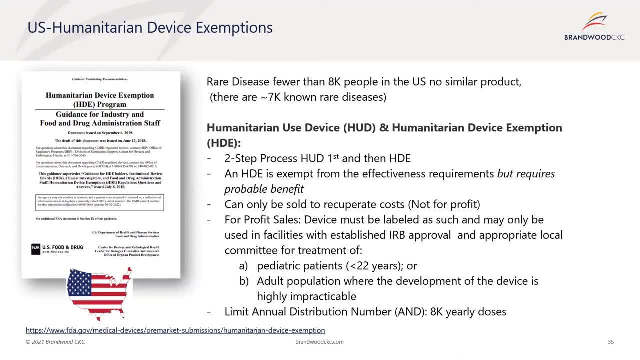 And what the FDA would really apply risk assessment to. the risk benefit met a ratio on approval of the product. There's not a full requirement that the product needs to be clinically validated, but that there needs to be a probable benefit, And I'll jump a little bit more into what that means with some more details. 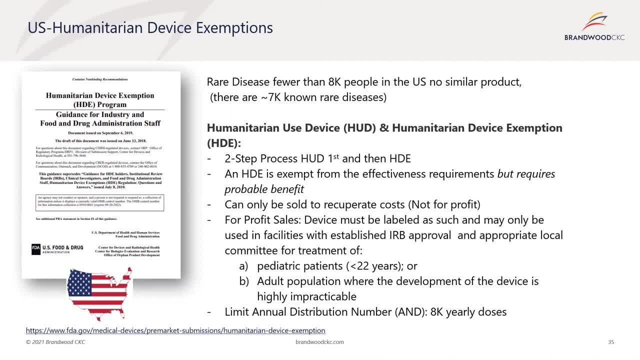 Here's some nuances to going down the risk, To going down the rare device, the rare disease device certification. It can only be sold to recuperate cost. There's a cap not for profit And, as of recently, there is a for profit sales module for these types of products. 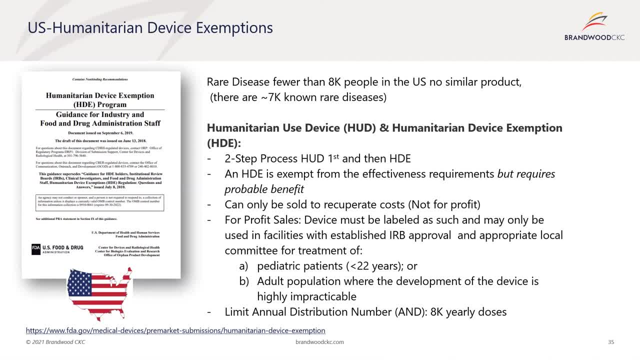 The device must be labeled as such and can only be used in IRB under IRB approval with an appropriate local committee for treatment, And the treatment needs to be for pediatric patients or an adult population where the development of the device is highly impractical. 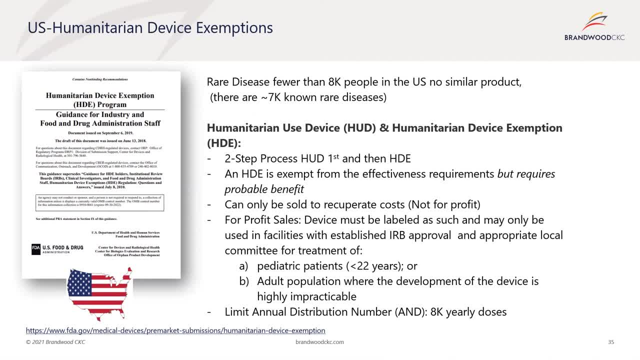 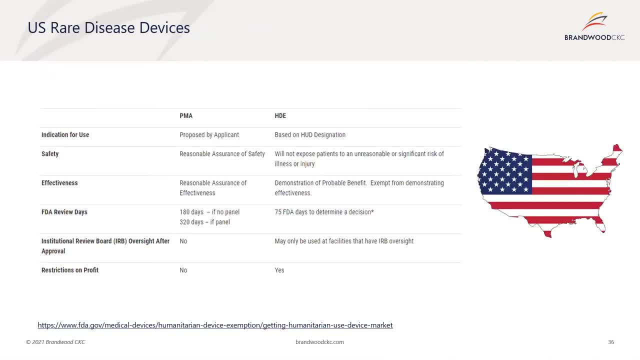 There is a limit of 8000 doses Annual distribution number on these products for profit. So if we compare the difference between a PMA and an HDE, the indication of use is proposed by the applicant with a PMA And the HDE is based on the HUD designation. 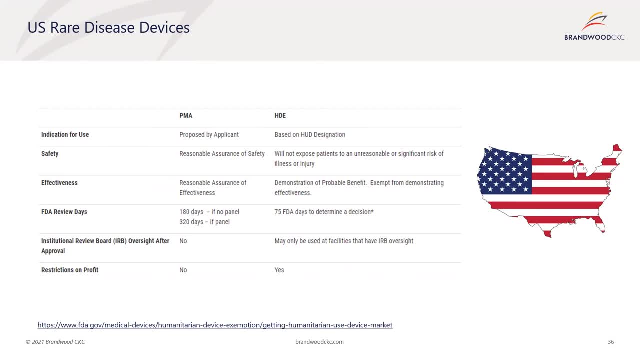 The safety needs to have a reasonable assurance for the PMA, And here's where we see a difference. It will not expose patients to an unreasonable significant risk for illness or injury. On the effectiveness side, of course, a PMA will require a clinical trial. 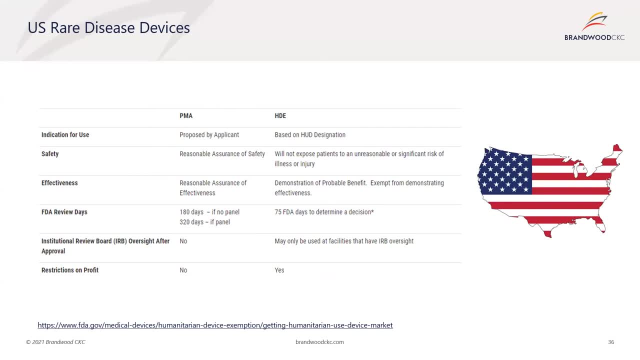 And here's what we're talking about. For the HDE, there has to be a demonstration of probable benefit And there is an exemption for demonstrating effectiveness. for the approval, The FDA review timeline is significantly smaller, There are restrictions for profit and the product can only be used under IRB approval. 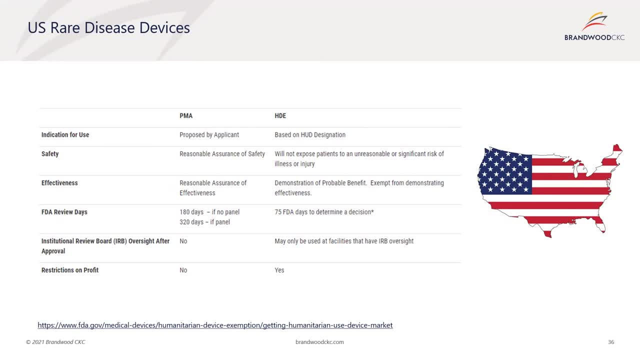 If we go on to those guidance documents, however, it does show the huge benefits that starting on a rare disease, not only talking about helping people's lives that don't have other options, but also about the benefit that generating early clinical data on a small patient population can do. 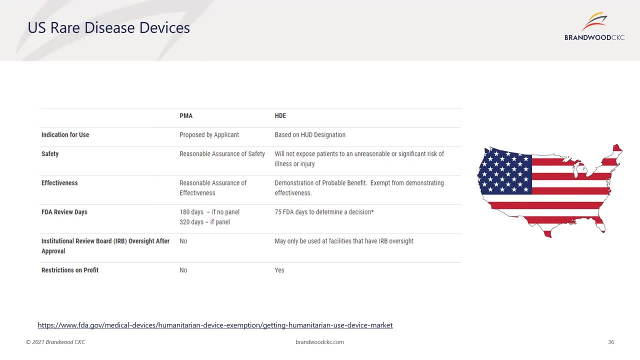 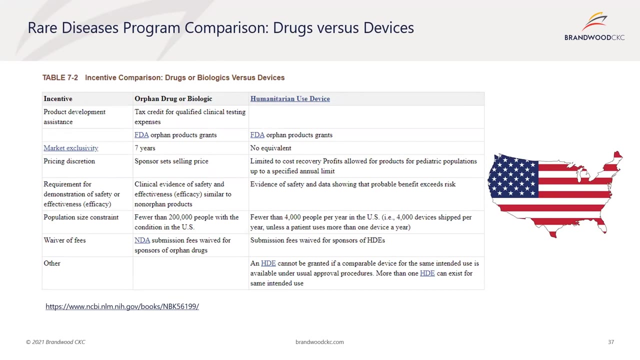 to then be leveraged, to then acquire a PMA or to accelerate the product development pathway, specifically also for pediatric applications. HDE tends to be a tremendous way to consider. Now, as good as the HDE program sounds, it's nearly as good. 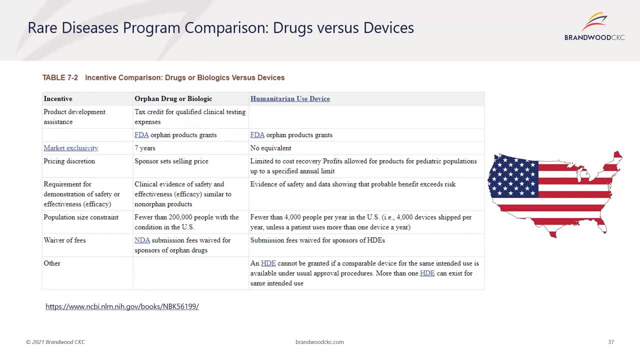 as an orphan drug or biologic sort of benefits, And it really is indicative of the cost, of course, of developing drugs versus devices. We know that the orphan drug- here there is an exclusivity for seven years. There's price and discretion. 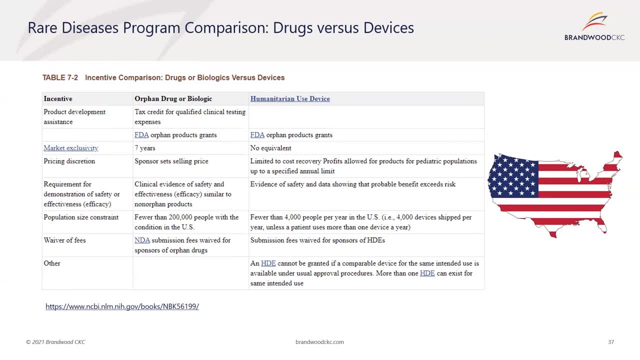 The clinical trial is somewhere. really. I guess a humanitarian use device does have significant improvement. There's clinical evidence of safety and effectiveness are similar to non-orphan products in the orphan drug designation And you can see the other areas where the comparison between orphan and humanitarian use devices maybe has still room for improvement. 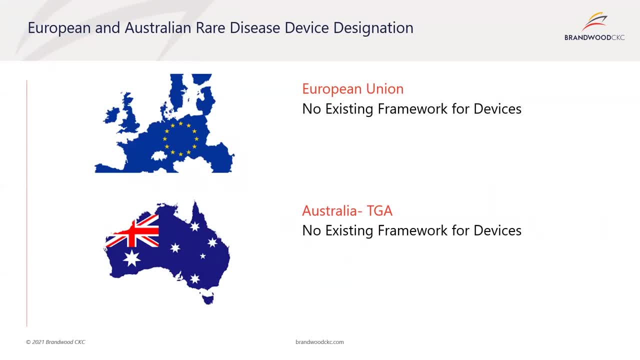 So if we were to ask: what's the position, What's the position of European Union? There's no existing framework for devices. The EMA does have a significant benefits for orphan drug, as we have outlined, very similar to that in the US. 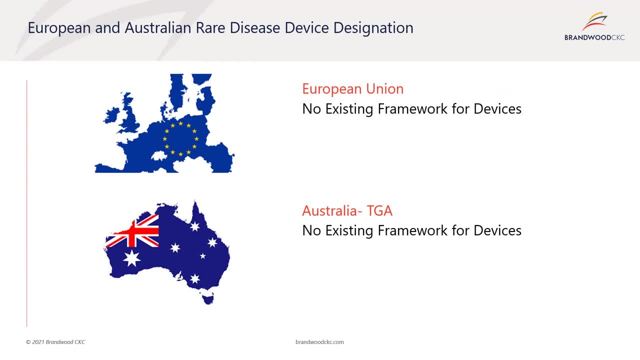 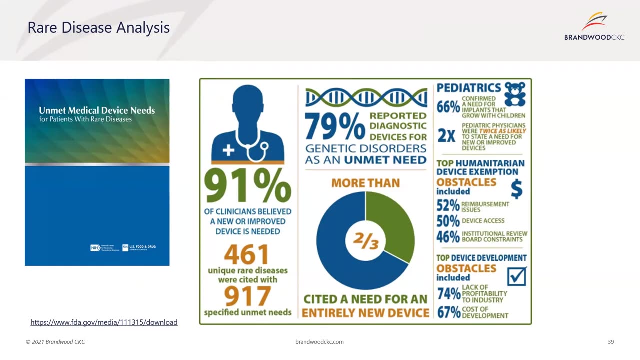 But there isn't something for devices. Now Australia is the same: There's an orphan designation for pharmaceutical products, but there isn't an existing framework for devices. I wanted to share this article, This NIH and FDA published report. They identified there's a significant need, specifically in the pediatrics. 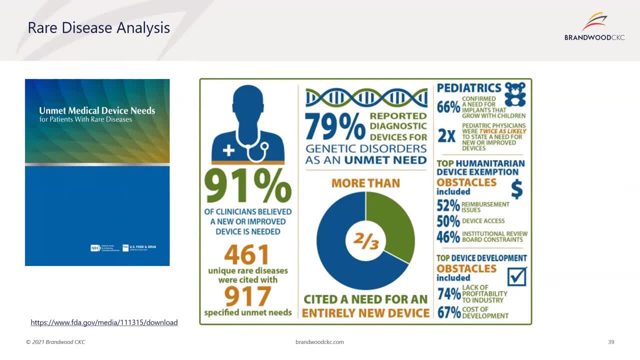 They need a 66% of our respondents of clinicians said that they need implants that have the capability of growing with the children as opposed to revision surgeries, And more than two thirds cited a need for an entirely new device For rare diseases. I mean, just the statistics are there. 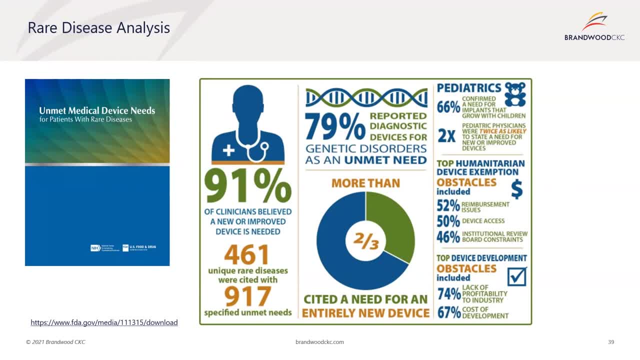 There's a tremendous need And I would say that innovative technologies can really see potentially find opportunities to bring products to market earlier to similar iterations for rare diseases and specifically for pediatrics. So I'm going to jump now into summary and conclusions. We covered a lot. 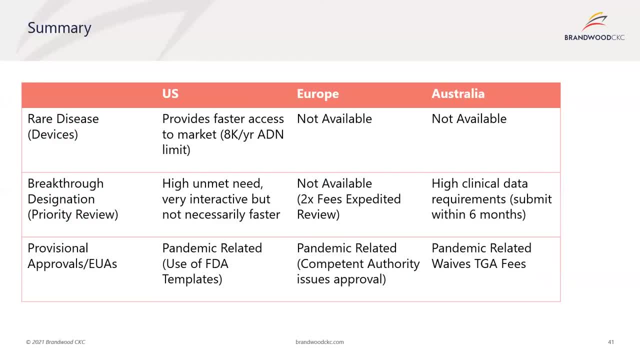 But some key points. I think this table really Summarizes Some key considerations Between the three Territories that we're covering today: The US, Europe and Australia. In terms of rare disease For devices, The US provides faster access to market. There's a limitation of 8,000.. Annual units per year, In terms of profit as well, But there's nothing similar in Europe and Australia. The breakthrough designation, The priority review: You have to have a high unmet need in the US. 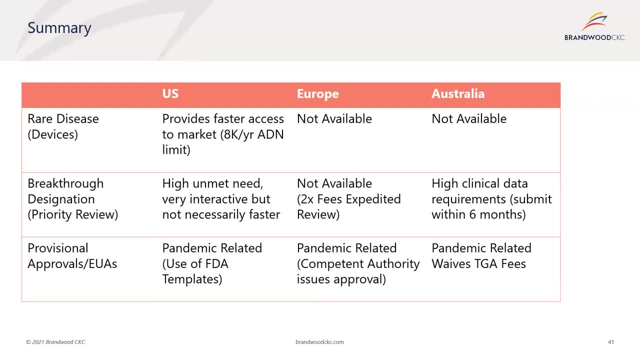 It provides you for a very interactive process. It's not necessarily faster- Currently The statistics don't Support that it's faster- But certainly The interaction makes it Very beneficial for the Developers In Europe. It's not available. 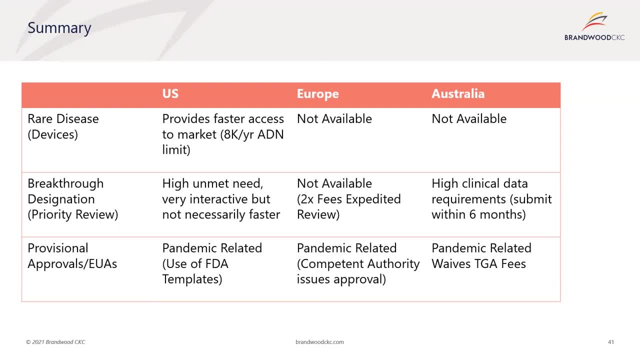 We'll see how many notified bodies Do adopt this, But under MDD There was ability to pay twice This year In the US It's not available. We'll see how many notified bodies Do adopt this, But under MDD. 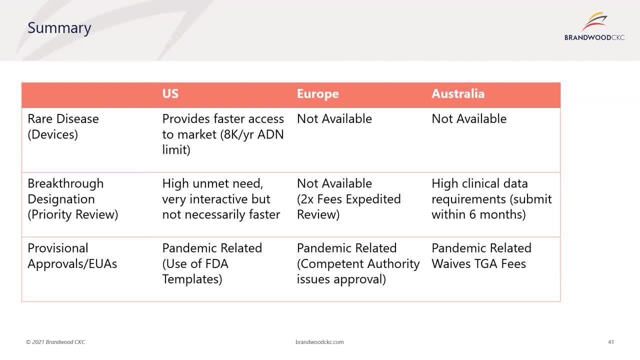 There was ability to pay twice. This year. It's not available. We'll see how many notified bodies Do adopt this. There was ability to pay twice This year. It's not available. We'll see how many notified bodies Do adopt this. 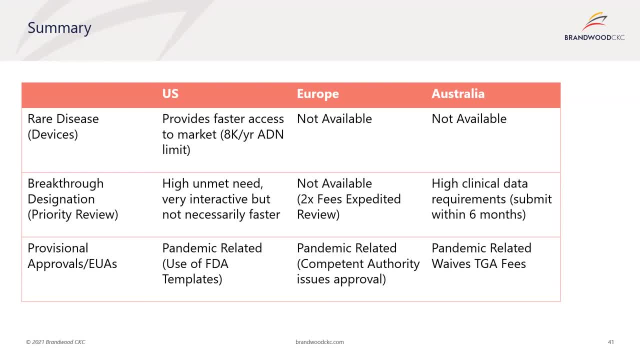 But under MDD It's not available. We'll see how many notified bodies Do adopt this, But under MDD It's not available. We'll see how many notified bodies Or do adopt this in the US It's not available. 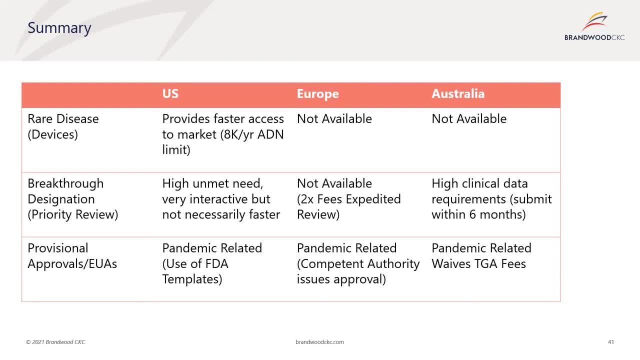 We'll see how many notified bodies. There was ability to pay twice The fees And get it somewhat of an expedited review. All right, You got that. The current backlogs- Probably MDR might not Allowed it In Australia. 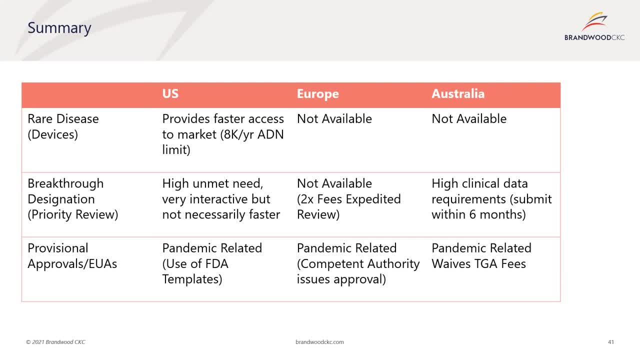 There is a breakthrough designation For high clinical data Required. but it does have high clinical data Requirements in a version use authorization. of course they have to be related to a pandemic in all instances. for FDA we want to say that the templates are phenomenal. 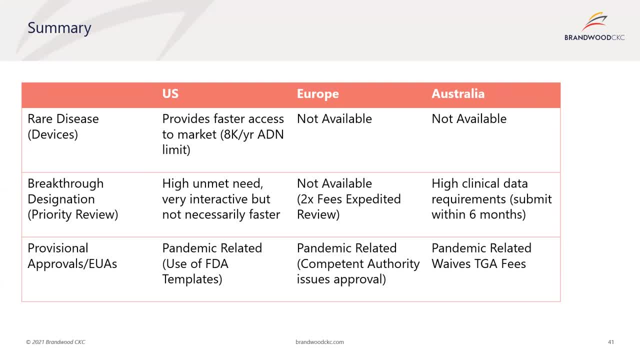 guidance on how, what the US will be requiring, and there are EUAs open for multiple modalities of treatment and diagnosis for COVID-19 in Europe. of course it has to be pandemic related, but you would work with one of the competent authorities, they would issue the provisional approval and that would. 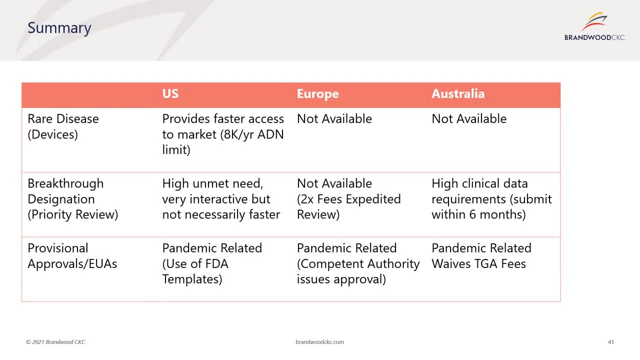 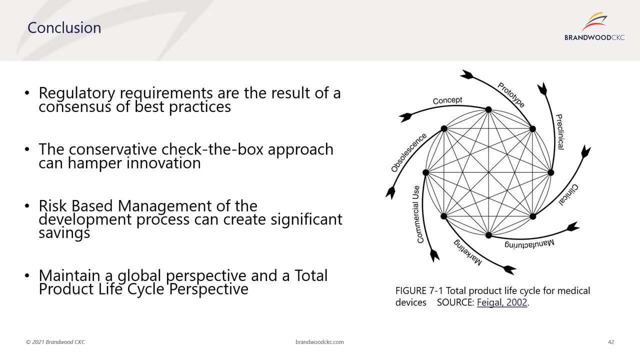 be then submitted to the other competent authorities in Australia has to be pandemic related and there's an additional benefit that TGA fees are waived or reduced. conclusion: regulatory requirements are the result of the consensus of best practices. so if we adopt that mindset, there certainly can be a change in the way that we treat COVID-19 in Australia and in other countries. so if we adopt that mindset, there certainly can be. 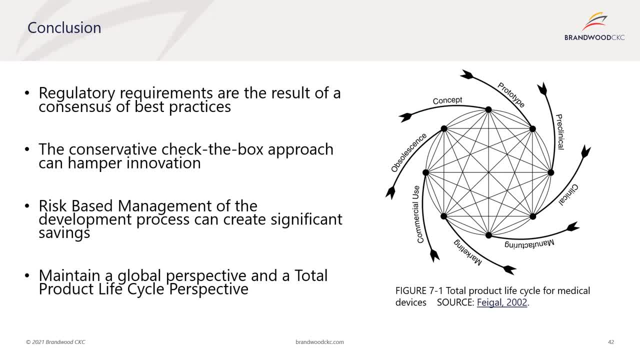 opportunities to apply innovative thought process and concepts to bring in innovative technologies to the market. I included this figure because it really emphasizes all the different aspects of the life cycle of a product and at each point there is room for innovative regulatory strategy considerations. we emphasize that the conservative check-the-box approach 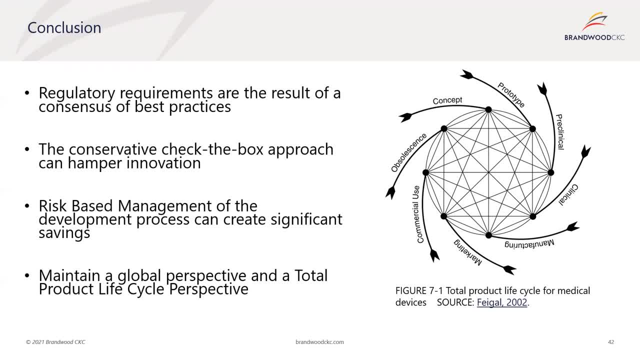 can really hamper innovation. it should be risk-based. there should be a lot of logic to what tests are done. the risk-based management of the development process can create significant savings and maintaining a global perspective and a total product life cycle perspective throughout the whole process of. 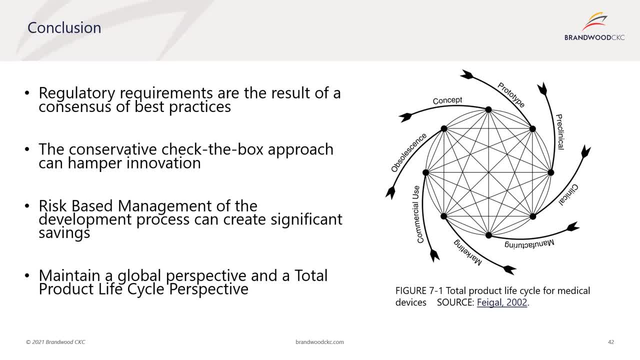 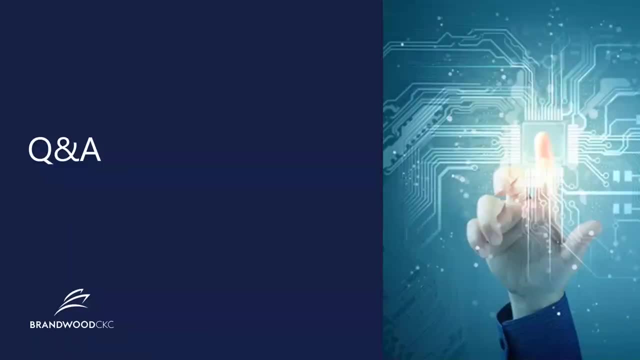 innovation, of bringing changes or new technologies to the market, can bring tremendous value for both the quality of life of patients and also for the manufacturers. so with that, I would say thank you very much for your time and I will see you in the next session. that I conclude my presentation, I'm going to address some questions that we 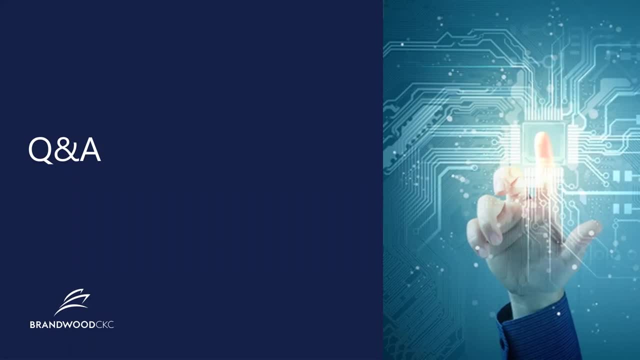 have received and we hope that you have enjoyed this presentation. so the first question. there was a question we were going to cover that: the novel pathway. can we elaborate on that? the the novel pathway is is somewhat new. the FDA sort of corrected their stance and that previously. 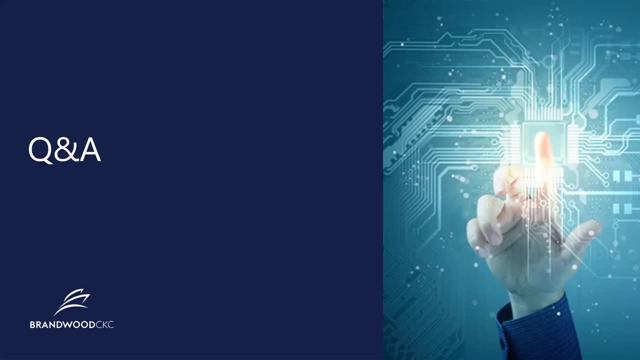 they had. there was a requirement to do a 510k and they get that rejected and then do the application and now there's a a way to directly apply for and request at an old classification. this applies to class 2 products. they are so innovative that there isn't. 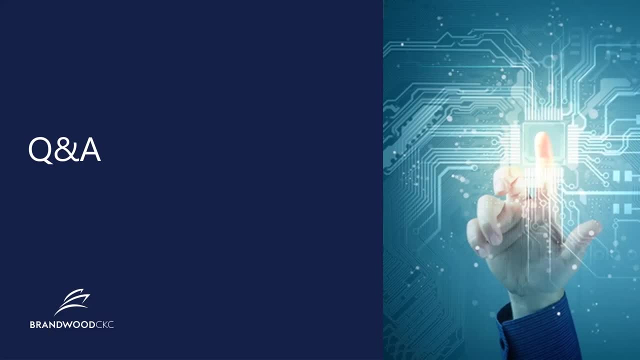 an appropriate code by FDA in the FDA database of a similar product. so, again for class 2 products, there is that pathway of the novel for innovative Technologies, and the FDA now has opened the application pathway for that determination to be done directly. there are some questions here. which trends do you anticipate in the next years in consequence of? 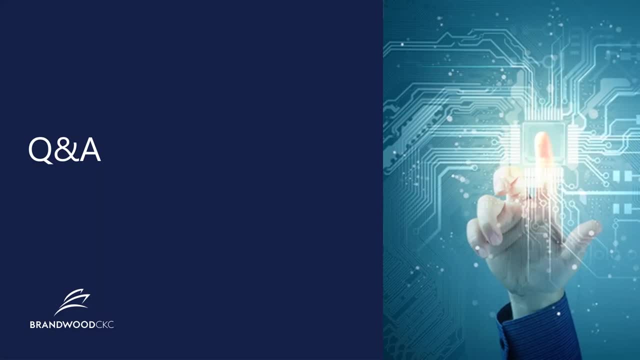 COVID-19. there's also AI, MDR and IVDR rollout and the increasing role of China in the medical device markets. we anticipate the diagnosis to be significantly improved in the breadth and depth of of its validations. many companies will be going through a 510k after obtaining EUA for COVID-19 and and that will just increase the robustness. 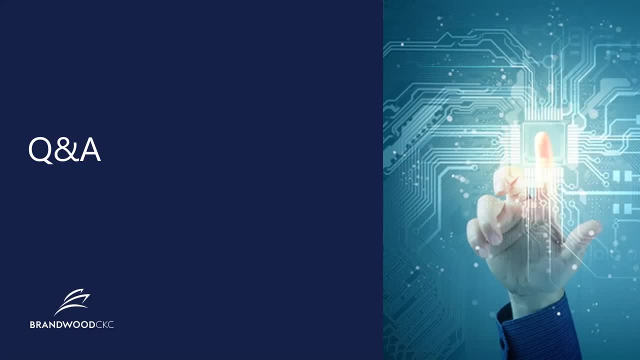 of, I think, the tasting testing capabilities. so I jumped first to the COVID-19. so we believe that's going to be a very positive for the diagnostic industry. in terms of AI, um, we have done webinars on softwares, medical device. there are noteworthy new regulations really now defining 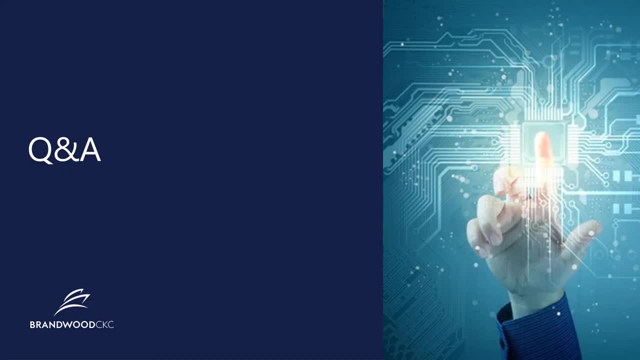 software's medical device that include AI, of course, and also software in medical device that include AI, both from the imdrf and also FDA and major regulars like TGA. I wanted to mention an exciting one, that's the center of excellence pilot program for software's medical device. 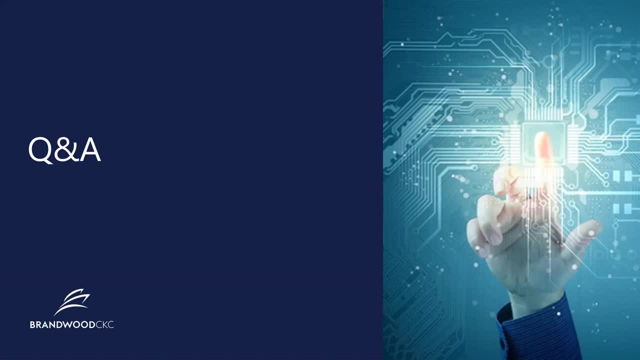 the FDA's pure heading. it's a phenomenal program in terms of the MDR and IVDR. we wanted to re-emphasize CERs and PRs and post-market surveillance are are the key really. um that that will be significantly improved in terms of what evidence manufacturers have there's. 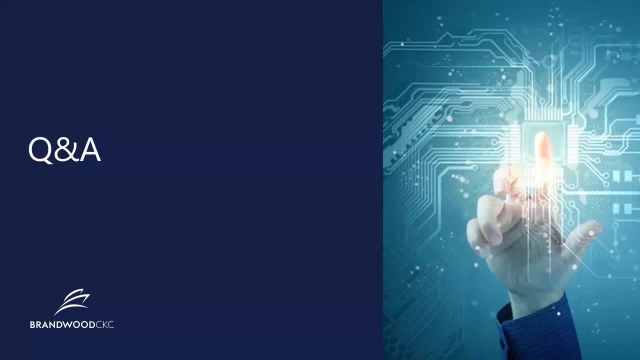 no grandfathering in of products, and so it's turning the the equation on its head. a statistic that really illustrates it, for example, for IVDRs: now IVDs will 90 to 80 percent of them will be have to undergo review by a notified body, whereas before 20 of them have previously only 20 been. 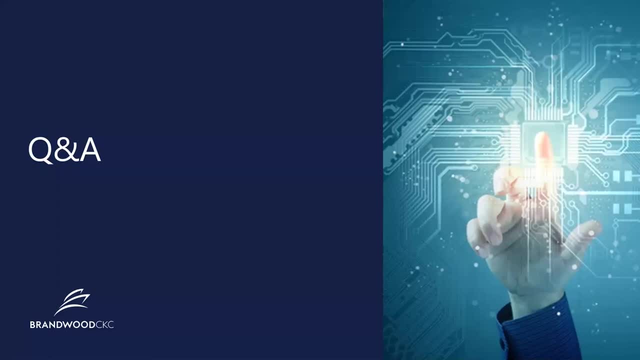 reviewed. China has recently issued new medical device mandate and this is, in theory, allowing new pathways to not require type testing, and there's also possible clinical trial exemptions beyond the exemptions listing, so that's a great progress in regards to China. now we also had a question on why the TGA is requiring a declaration of conformity.